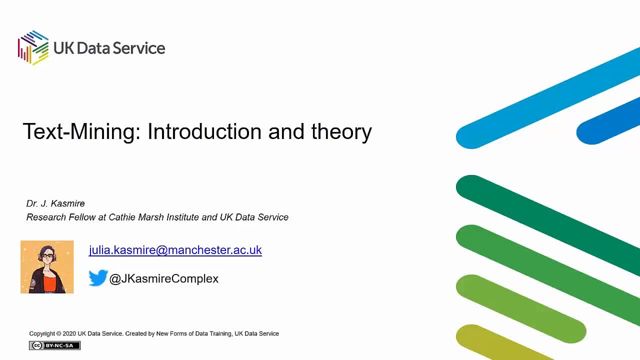 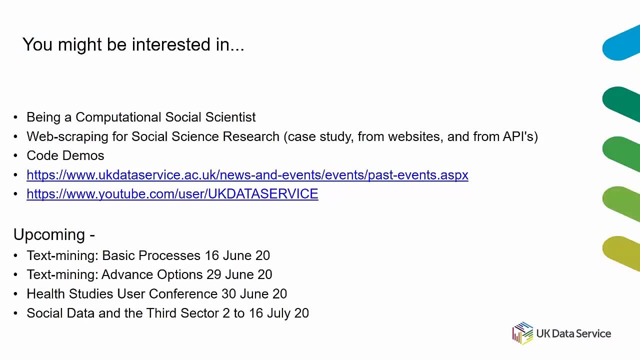 This is text mining and introduction and theory, So we won't be doing any coding in this webinar. but there are two more webinars you see here in the upcoming section: Basic processes on the 16th of June and advanced options on the 29th of June. I will be demonstrating code in both of those webinars and I will also provide you with Jupyter notebooks so that you can work through the code on your own or copy-paste into another platform as you like. 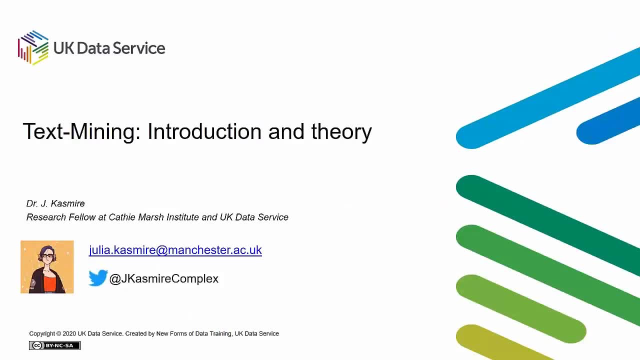 So before we move on, I'll just say my name is Dr Julia Kazmaier. I'm a research fellow at the Cathy Marsh Institute in the UK Data Service. Please feel free to send me emails or tweets about questions you have about this webinar or any other work that that you've seen me do. I'm happy to engage with the topics on various platforms, but diving into the topic today, 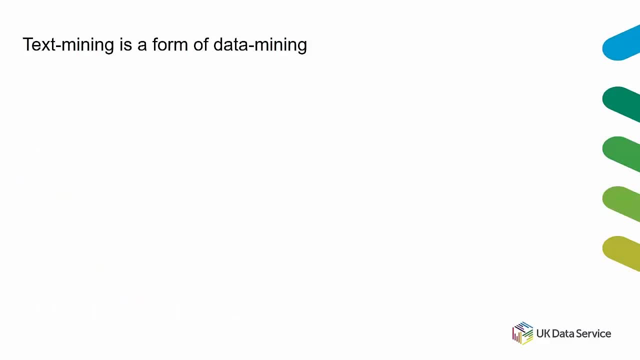 Just want to start out and say text mining is one kind of data mining that, as you might have guessed, looks at text. That might seem blindingly obvious and that's fine, but we're going to dive into that a little bit more. 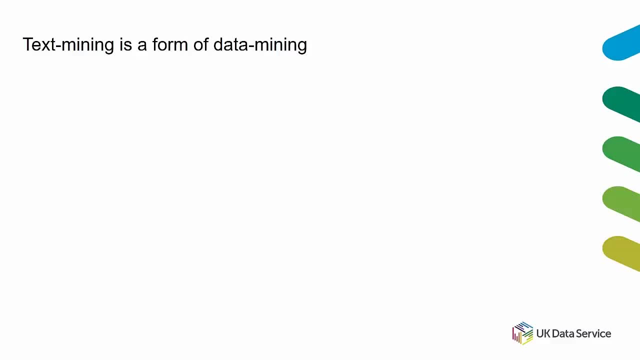 And maybe uncover some things you wouldn't have thought about. So other kinds of data mining might look at images and sound movements. you know lots of other kinds of data out there And we may do webinars on those in the future, but today we're just focusing on text mining. 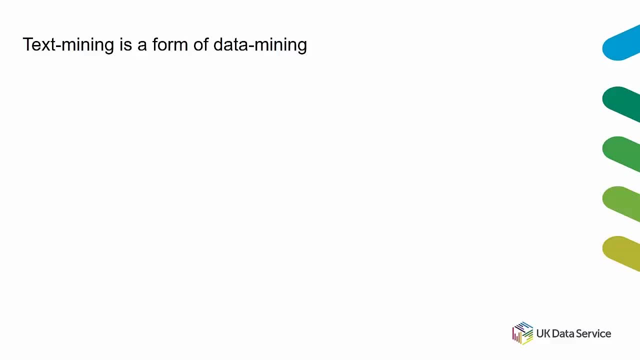 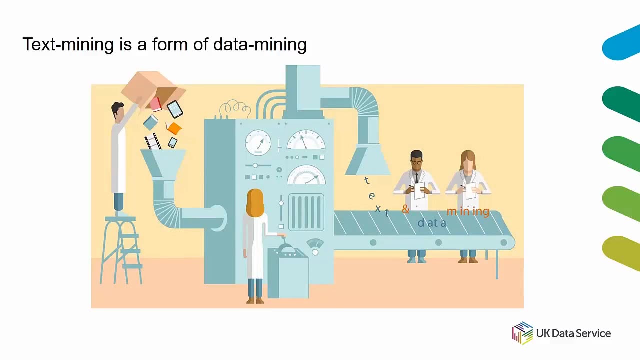 But importantly, data mining, or indeed text mining, is not just a buzzword. It's actually a large category of research methods based around the idea of transformation. Stuff goes into one end of a sort of transformation machine and it comes out. 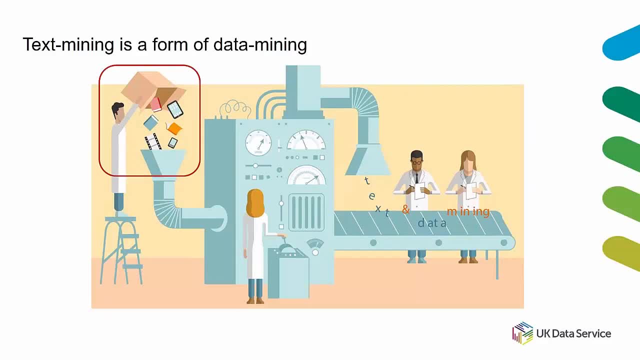 you know at the other end. But what is it that goes in and what comes out? Lots of things can go in: Text, obviously, But also recordings of speech, videos, images, you know, seismographic information. who knows Unstructured data, usually in chunks? 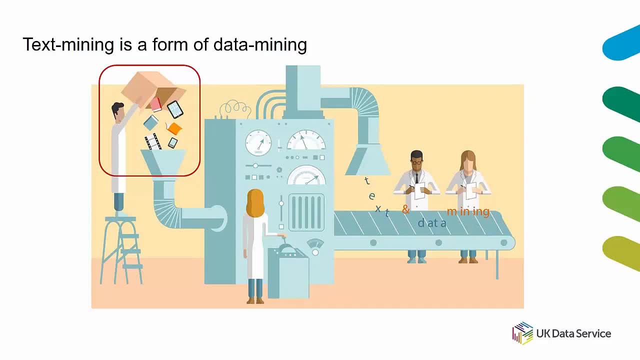 Things could be like a blog, which is an unstructured sort of relatively unstructured chunk of writing, But also, you know know, images or live video feeds. it's because it can also be a stream as well as chunks. so what comes out of the transformation process? well, data. 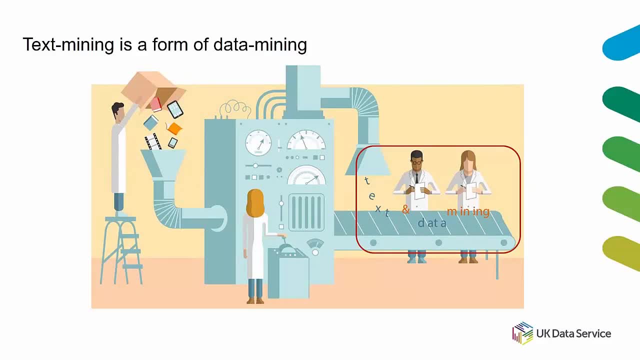 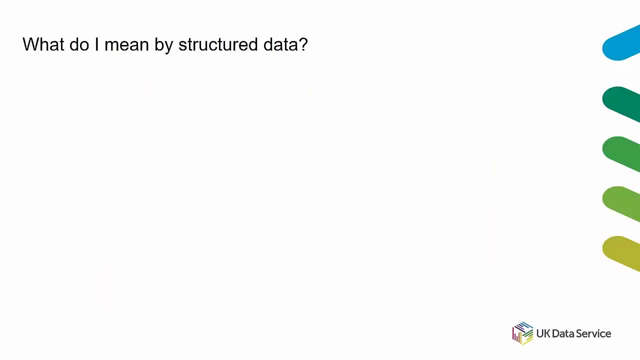 specifically structured data, and let's talk a little bit about that. so what do I mean by structured data? well, I mean most people. when they think about structured data, they think of the kind of that data that comes in databases or excel sheets, vectors or arrays or a matrix or something like that. they're 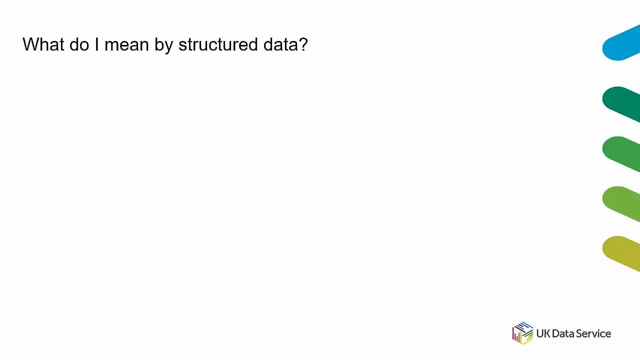 arranged in structured ways, usually depicted as rows and columns or as tables. for example, if I want to track my online education sessions, I would probably want to record basic information like the title of the session I gave, maybe the date I gave it, the number of attendees: 75. there are. 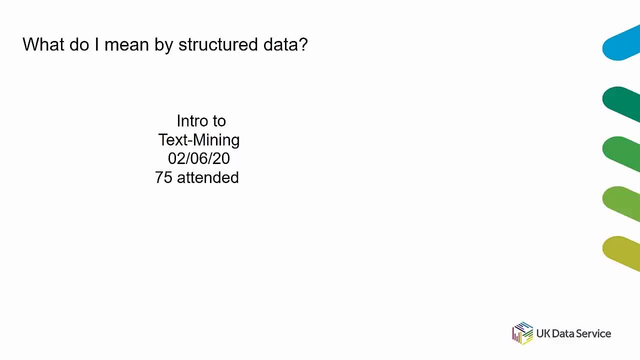 actually much more than you, than 75 attending, so that's great. thumbs up to all of you. now I could write this information on a sticky note and tack it to my cardboard, and that is indeed how lots of people record information. but if I can assume that I will be, 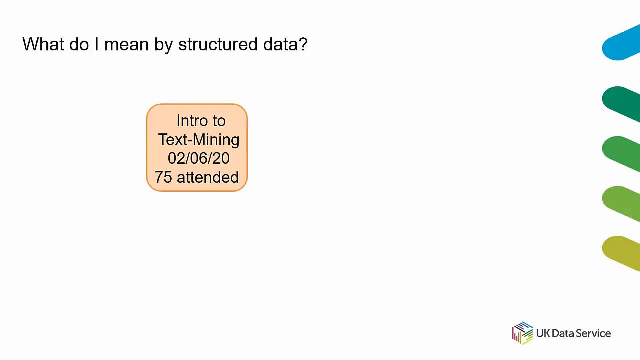 giving lots of online education sessions. it's probably safe to assume that I want to do something a little bit more interesting than just tack it to my corkboard. I might want to calculate my average attendance or plot whether my sessions are becoming more or less frequent over time. might want to you. 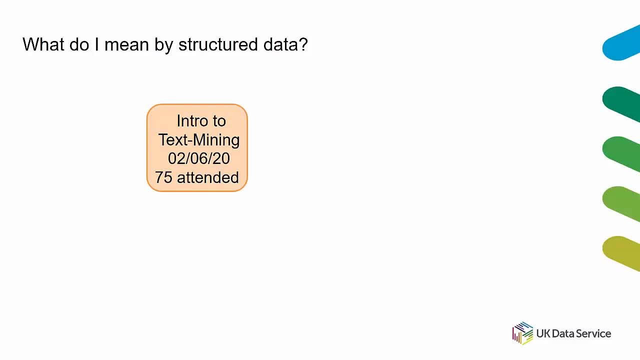 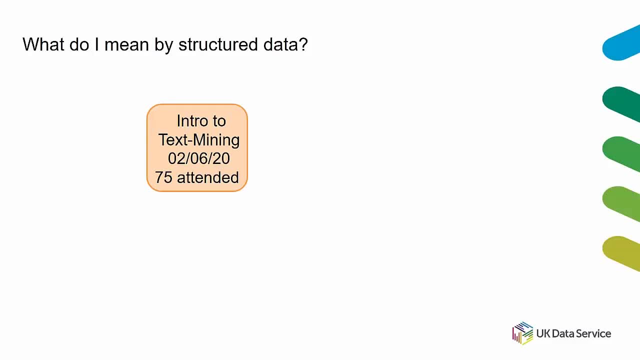 because I want to make sure that I'm paying attention to the volume of data. so, knowing this, it's much more sensible to record this data for a given education education session in the same place and in the same order as the other information that I collect on other education sessions. so you know, obviously. 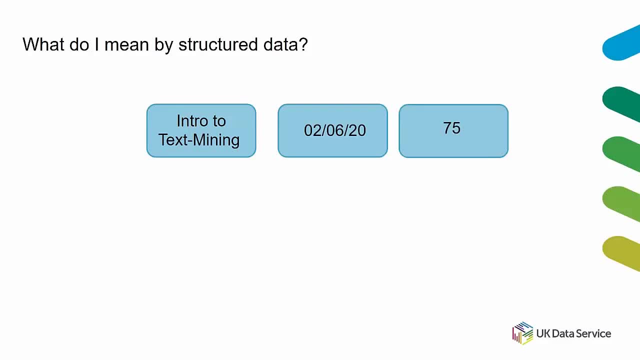 I can do better than sticky notes. tack to my corkboard. I can, you know, sort of in rows and columns. so you know this is back to Excel spreadsheets or data mining or sort of databases and arrays and that kind of thing. now, if I do this, 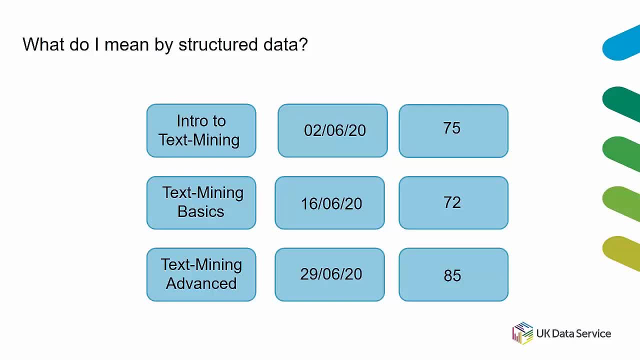 for each, all the different sessions, and I can have the same format in each column and same related content in each row. so in the columns- this column, for example- I have all the titles, and this one all the dates, and this one all the attendance, and in the rows are all things that relate to each other. so this: 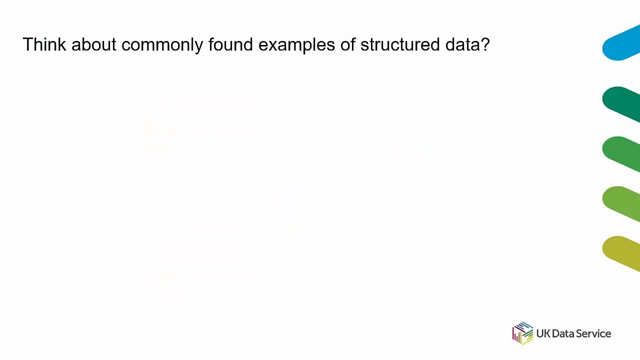 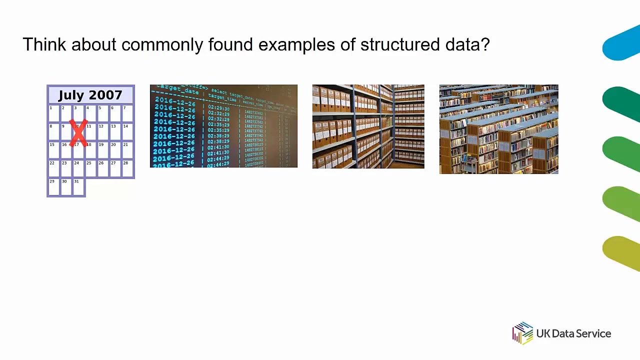 title and this date and this attendance are all for the same event. now it's pretty obvious. I think we all you know we're pretty good with it, stuff like that. but there are maybe less obvious examples of structured data. so calendars are structured data because they're in rows and columns for days of the week. 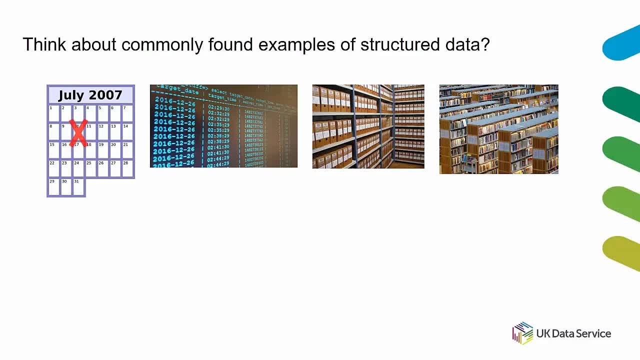 and you know sequential order database systems, obviously very, very structured, but not necessary in rows and columns. there can be tables and sort of linked tables and dictionaries and things like that filing systems. obviously quite structured libraries, but also less obvious examples like a grocery store where things in the 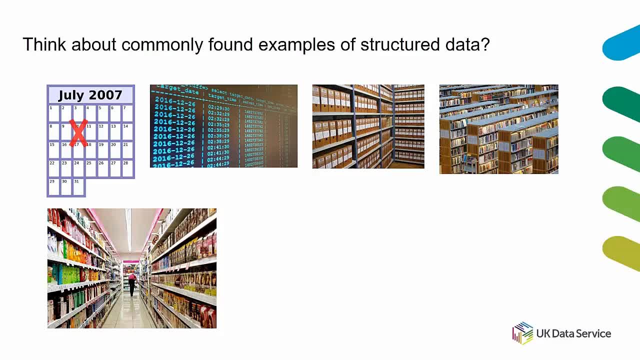 aisle, at least in principle, go together or share something in common: your wardrobe, where hopefully you don't have, like, your business suits, and your hiking boots and your underpants all shared with you. and then the other thing I would say is that you need to make some. 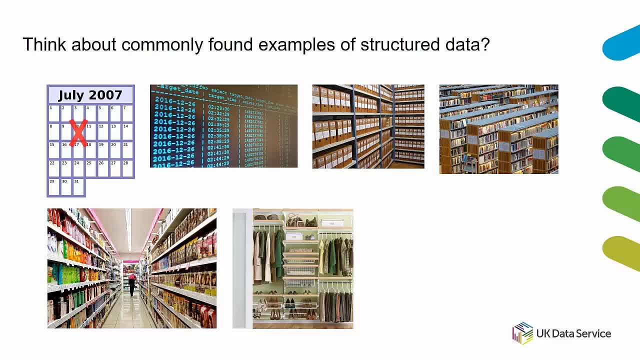 shoved into the same drawer. instead, you have them structured so that they're things that need to hang or hanging and things that go together are all in the same drawer. also even train stations, because the platforms are structured and the people move in certain ways and the information is is shared out in in. 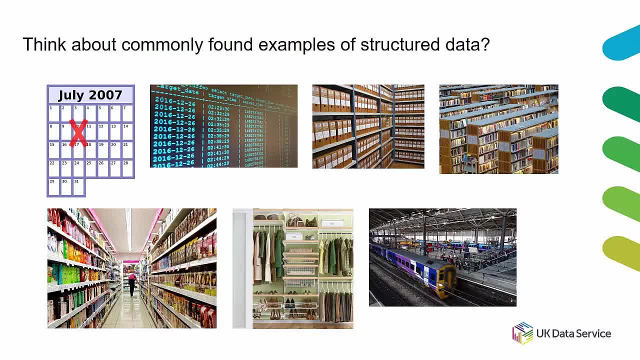 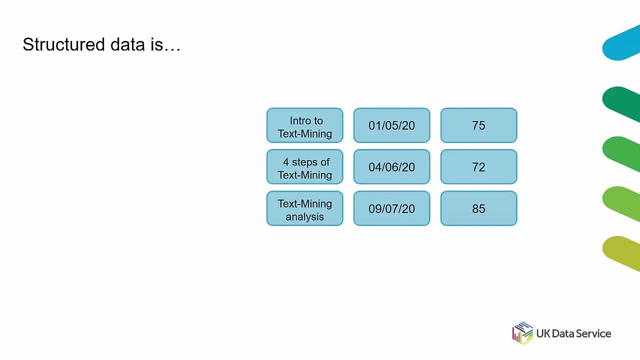 structures in an organized fashion. so these are maybe less obvious examples of structured data. so the thing about structured data is from a statistical point of view is really familiar. it's really easy. it's really easy to demonstrate how to work with it and how we came to the conclusions you know for 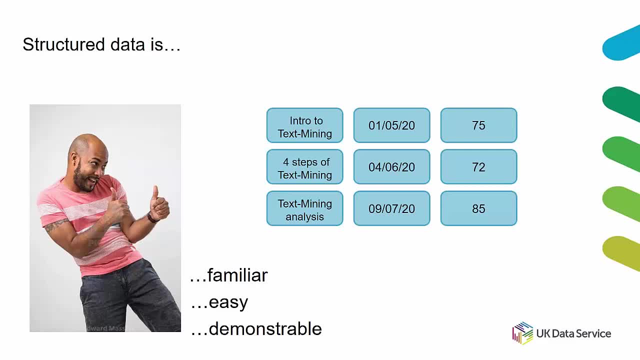 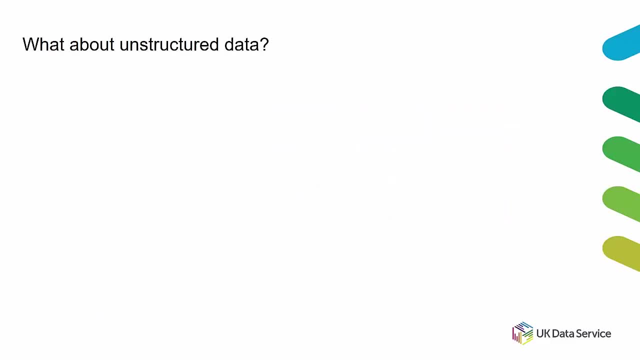 example, if I wanted to show what the average attendance was for these sessions. it's easy to see that you add up the columns and divide by the number of columns. that's great, but what about unstructured data? now, this is very familiar to us in our lives. we move through a world in which data is largely 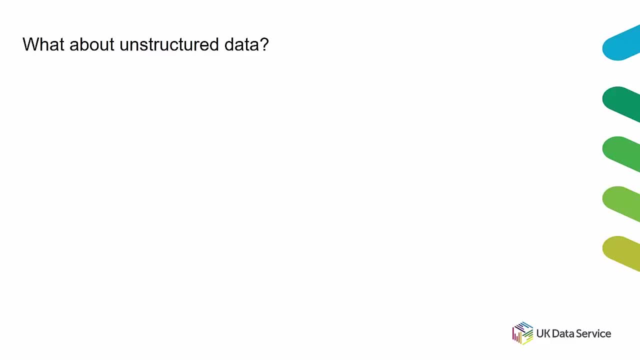 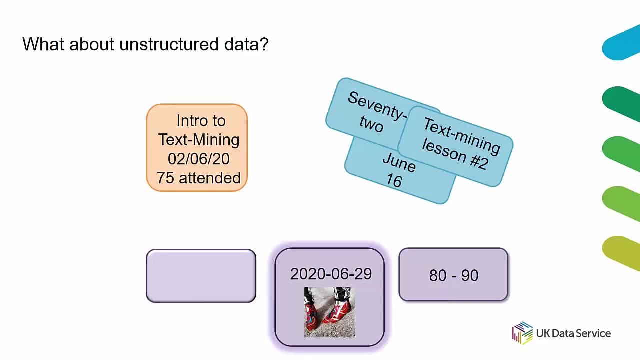 unstructured, but it's less familiar or easier or demonstrable to work with in the way that data scientists are used to working with data. the actual information is probably about the same, but the lack of structure means it's all jumbled up together in one document like this. first, 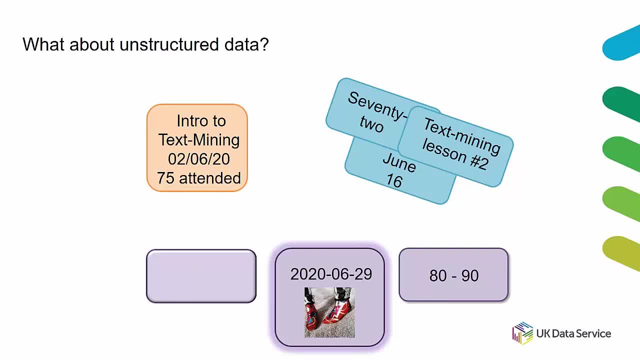 one it's. it's all put on one sticky note. but in the second case it's on three different sticky notes, and in the third case, you know, some of the information is missing. so here it's all jumbled together. here it's, it's the same. 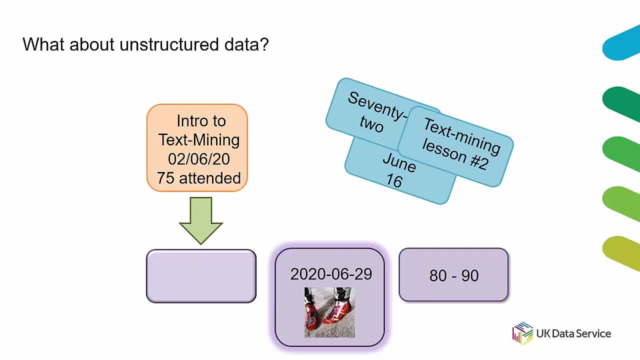 information, but spread across three different notes. this one's missing a title. I have no idea why. I must have lost the sticky note also. things are in a different format, so I've written the dates here in three different ways. I've written the people who attend in. 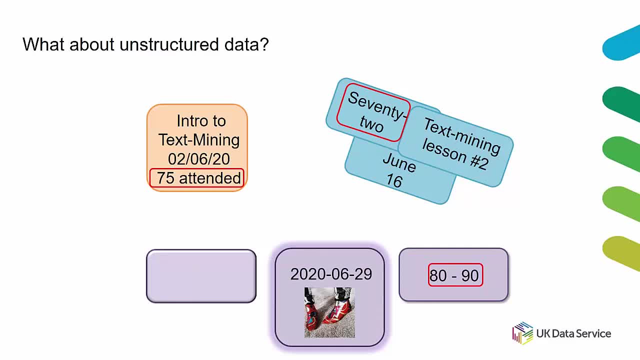 three different ways. one is a key value pair, where 75 is the value and attended as the key. one is written out. the numbers are written out, but there's no key. and then one is even a date range- sorry, a numerical range, it's not, not a. 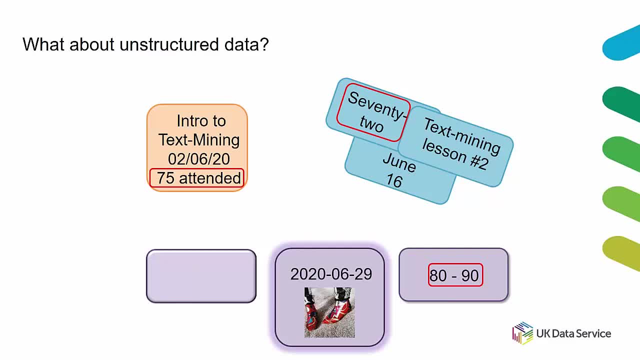 specific date, it's all just a name. as you can imagine, right now there's no date, also no key, so that you know this is more or less the same information, but in a very unstructured, inconsistent way. now that's that can be a problem. there's. 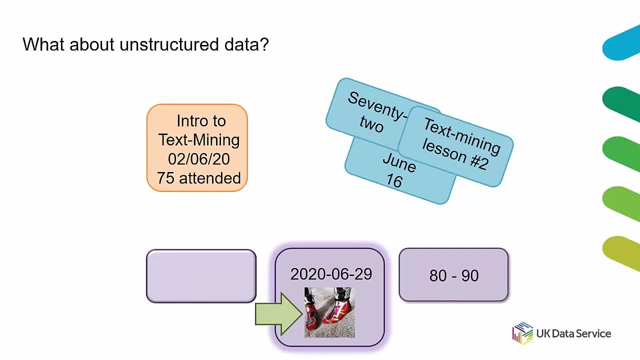 also superfluous data, like this picture of the shoes that I was wearing, that I want to wear when I give this session. you know they're great shoes, but doesn't need to be there. so the key point to take away when you're looking at unstructured data is actually that it's semi structured or semi unstructured. 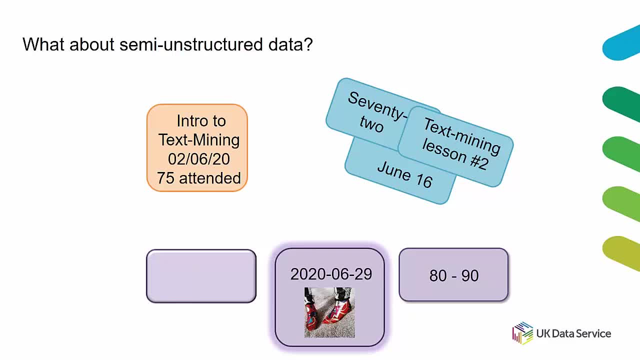 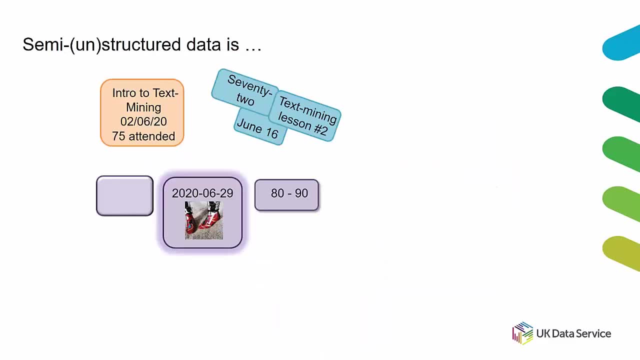 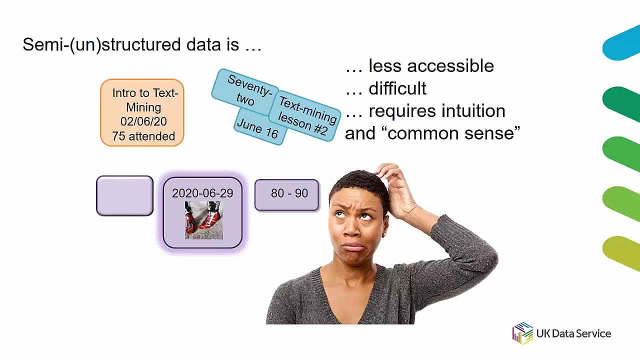 there's still a lot of structure here, but the structure is less coherent and order and orderly and tidy. it's less immediately accessible. so in this case, semi structured or semi unstructured, depending on how you know whether you're a glass half full, a glass half empty kind of person is less accessible. it's. 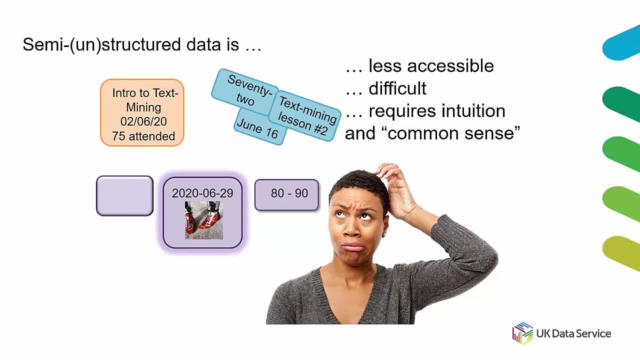 difficult. it requires a lot of intuition and common sense with how to work with it, and intuition and common sense are not really available to computers. so trying to get a computer to do this is very difficult. but that's fine, because that's what text mining or data mining is about. so it is. 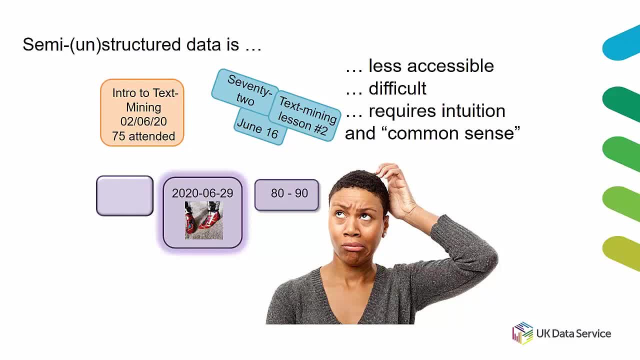 important to say that historically, like intuition and common sense, can be applied to unstructured or semi structured data. that's fine. it just means that sort of getting insights and conclusions and results out of working with this kind of data requires a lot of time, a lot of expertise- developed slowly- a lot of gut instinct, and that when 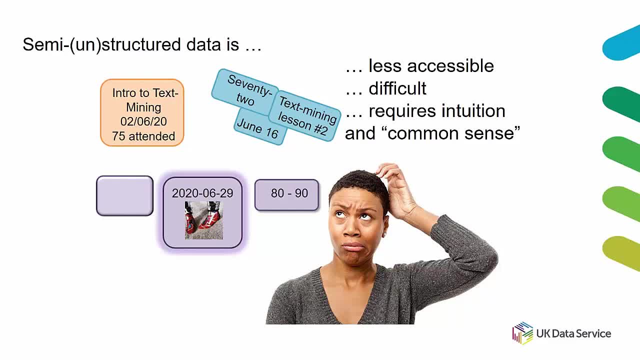 people you don't want to share their conclusions. it's really hard for someone else to reach the same conclusion because it's such a slow and difficult and personal process, so it's hard for you to share that with other people. that's why I'm doing this. 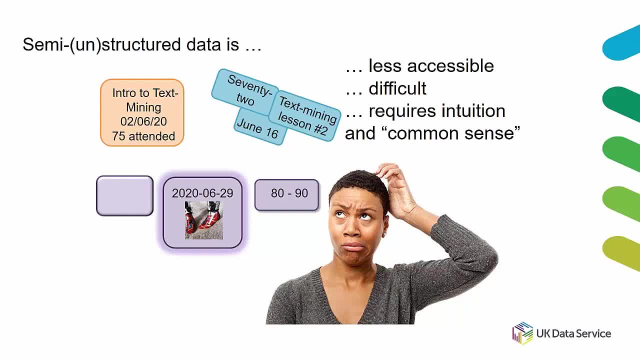 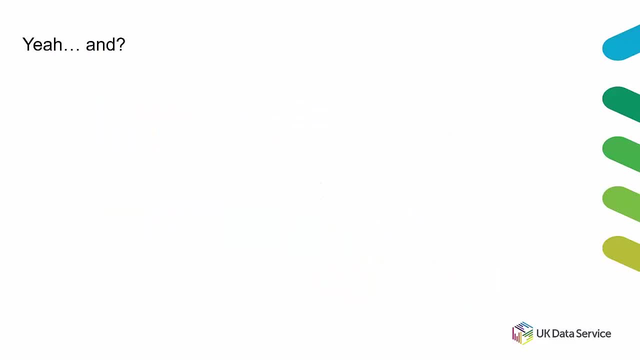 your work. it's hard to show how you came to your conclusions, hard to convince someone else to come to the same conclusion. It's a little bit difficult and that's why you know certain historically scientific sort of things that worked with structured data. you know temperatures and dates and 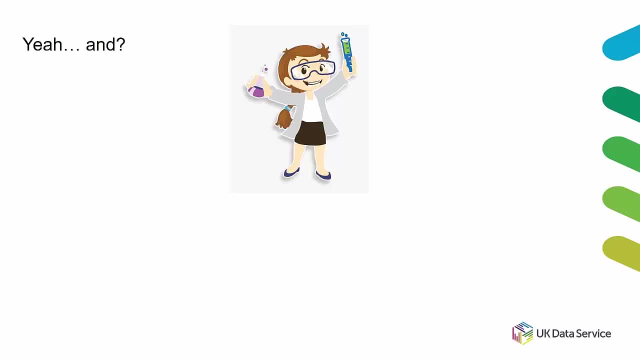 numbers, different kinds of values that can be recorded in a very structured way. People can show their work and they can publish their results and it's, you know, easy to see the conclusions, whereas, you know, humanities had a lot of discussion and interpretation. 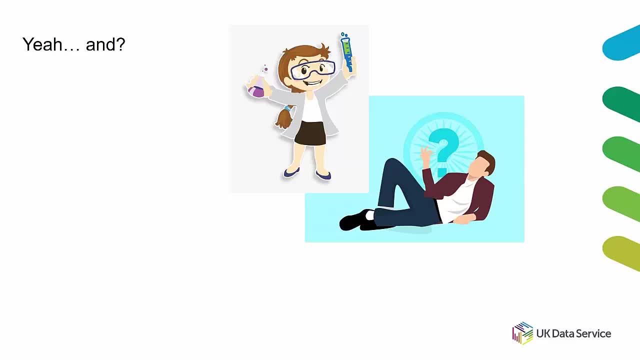 and you know the work. a humanities paper tends to have different sections than a hard sciences paper, for example, because just showing the work is difficult. So why does this matter, though The division? it used to be that we just gave structured data to the sciences and unstructured 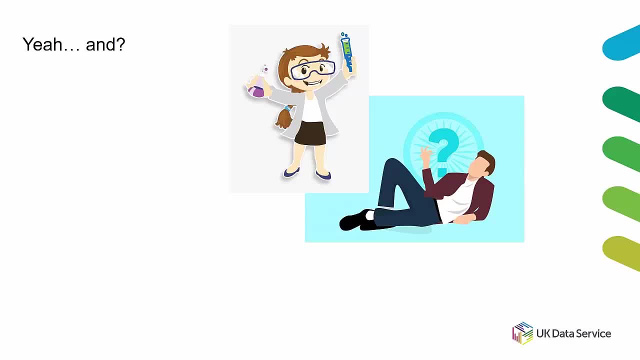 data to the humanities And people just did separate work on separate kinds of data. Well, that's not entirely great, because the division is getting a bit boring and really we don't want to limit ourselves in how we approach things, especially in a world where 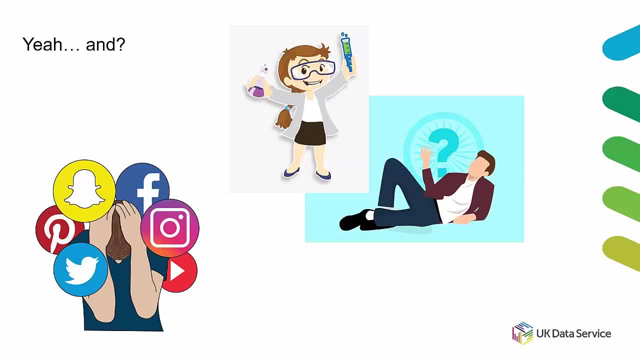 semi unstructured data is now absolutely everywhere around us. you know social media and fitness trackers and geolocation data on your phone And there's all kinds of data that is kind of structured And it says something about how we live our lives, but it's hard to work with in traditional 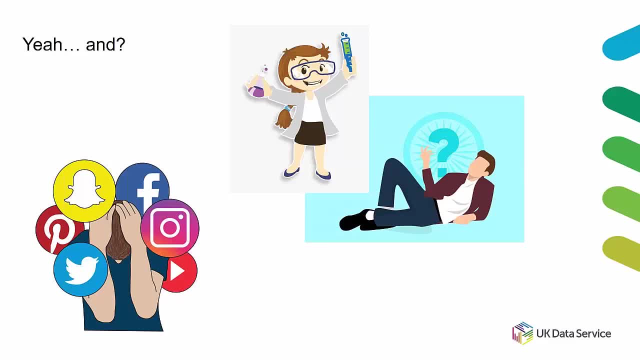 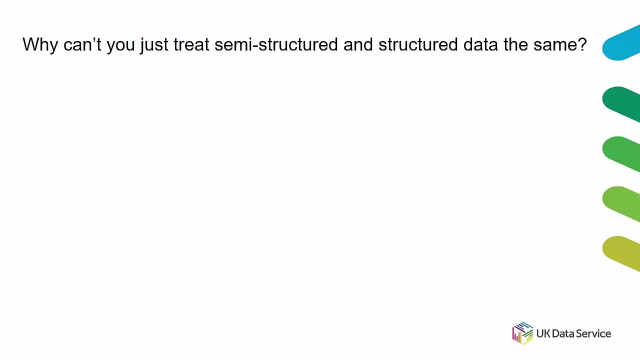 ways, It's also happening much too quickly to become an expert on, in the traditional humanities approach of sort, of reading all that there is to read and thinking critically about it, writing another book. So what are we going to do? Well, you can't just treat them the same. 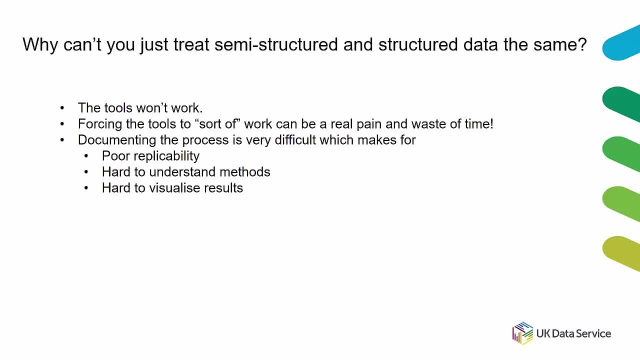 You can't because the tools just won't work. You can't. You can't force a blog into you know an Excel spreadsheet and expect to do anything useful with it. It's also the process of forcing it into an Excel spreadsheet is going to be really difficult. 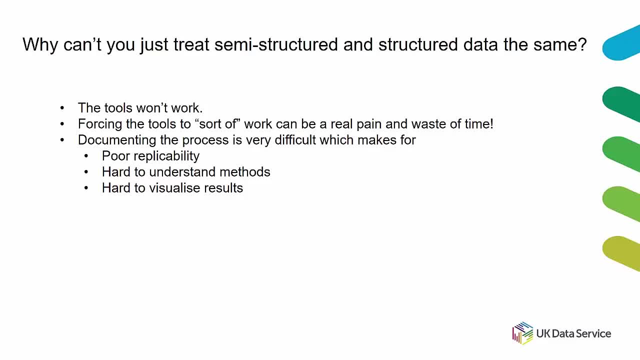 It's going to be a waste of time. It's it's not going to be easy to describe how you did that or why you did it, So no one else will be able to replicate your work anyway. First, you need to turn the semi structured data into structured data. 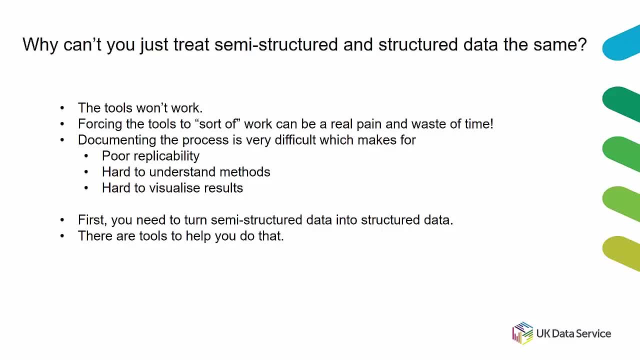 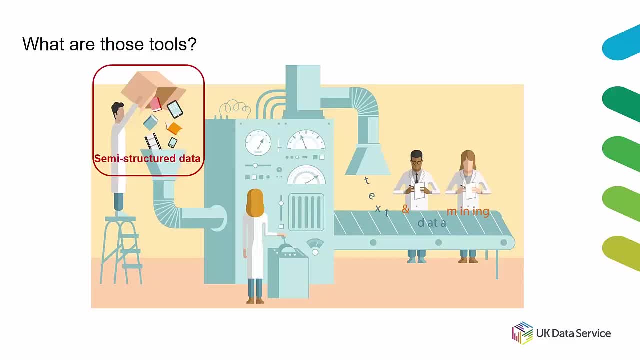 And there are tools to help you do that, And I recommend you use them, which is what we're going to deal with now. It's just a quick look back at this image, like what goes in is semi structured data and what comes out is structured data. 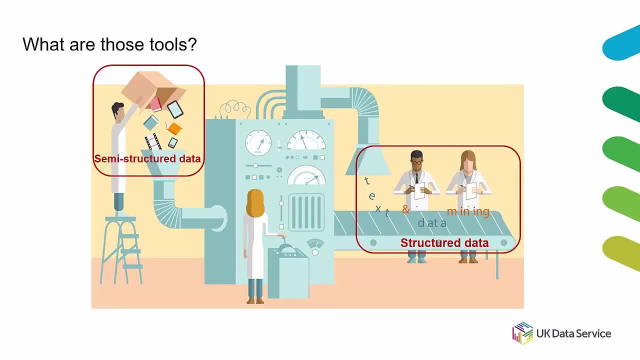 And the machine that does this transformation is, for our purposes, text mining, but it could be data mining more broadly. And it does that by capturing the structure that already exists in semi structured data and amplifying it And cutting off the bits that don't fit into the, the amplified structure. 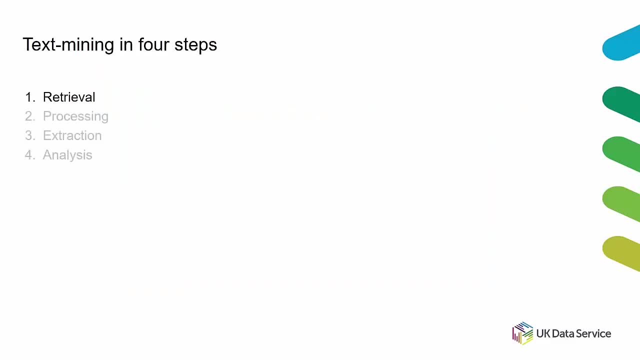 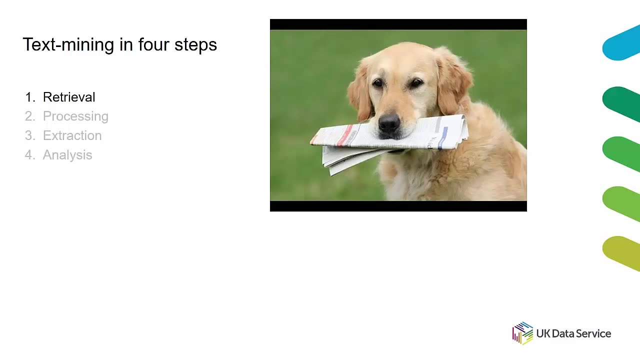 There are four basic steps which I will walk you through now. The first is retrieval- And you will be familiar with this if you watched any of our web scraping webinar series- because it is about acquiring data so you can scrape it off the web or you can download. 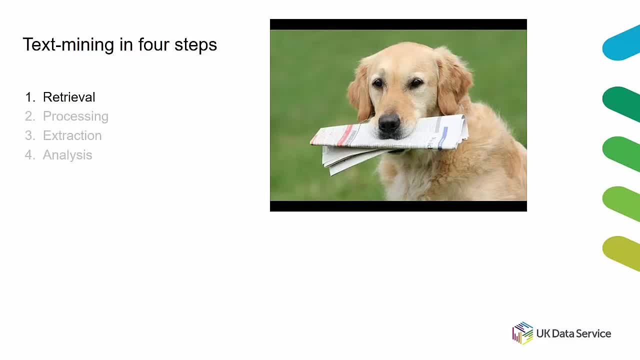 it through an API Or, in fact, you could, you know, digitize some records from the local database. There's a lot of different ways you can acquire data, you can retrieve the information to work with. So, for example, let's say that I want to identify some language that politicians use when they 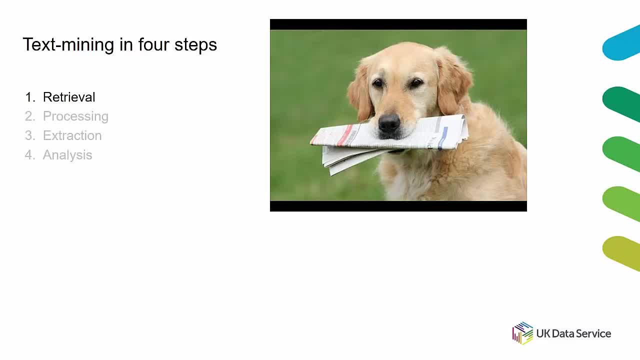 are talking about projects that are unlikely to actually get off the ground, as opposed to projects that are very likely to genuinely happen. So first I would want to retrieve a set of texts that include speech of writing about projects from politicians about projects, And that must include some that I know that happened and some that I know didn't happen. 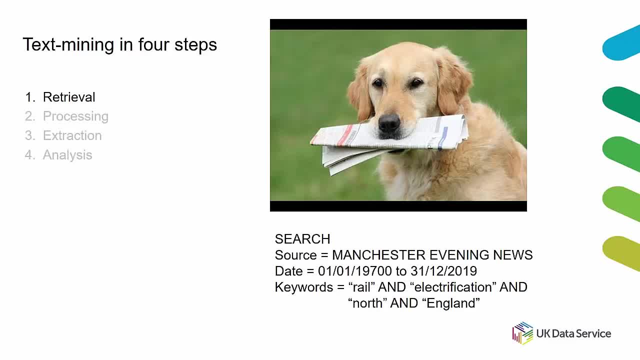 And I might, for example, do a search through LexisNexis or some kind of like news source search engine and, you know, specify a source and a date range and keywords to look at. In this case, rail electrification in the north of England was the topic I was looking. 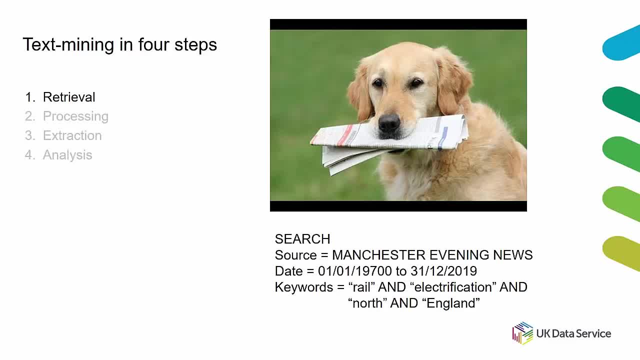 at And I want to sort of get- Okay, You know, at least a hundred or a thousand or something like that- texts in newspaper articles, in this case on this topic. that would be a good retrieval method for getting text to work with with text mining. 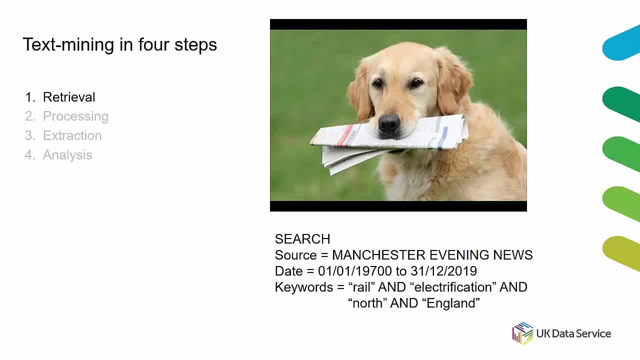 Now I would also want to have some projects that I know were successful, but this is just an example of the kind of thing I see a typo in the date range. that is not going to help Anyway, so it's always preferable to keep a copy of your raw acquired data. 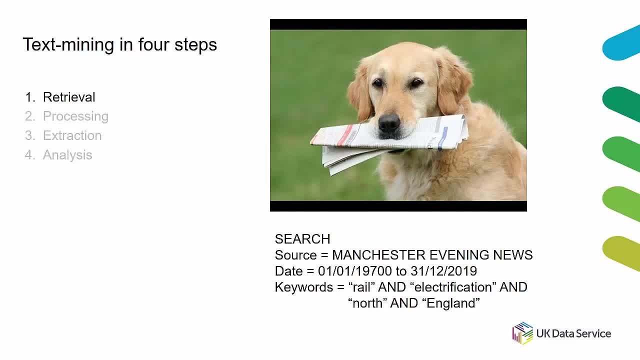 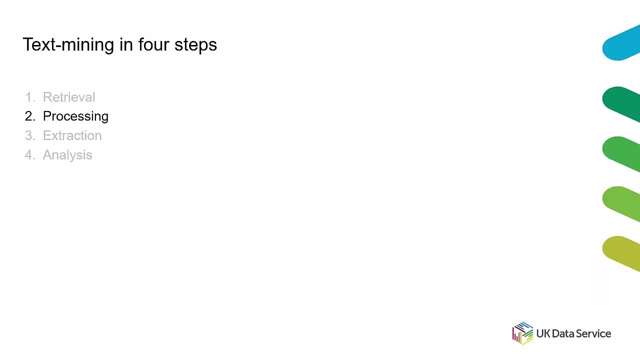 So, whatever you get from this search, you run this search, download a big data file, always keep that separate and work through the rest of the steps on a copy of that data. That way you can provide your raw data for anyone who wants to replicate your steps. 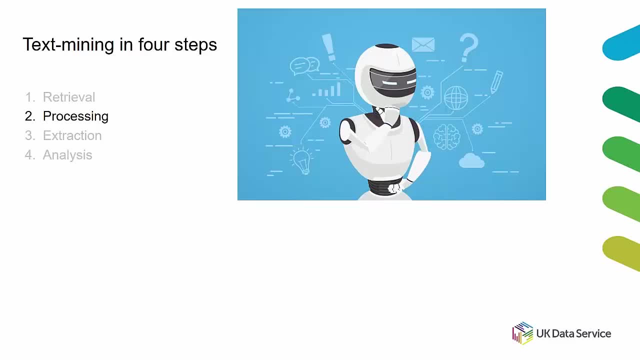 The next step is processing, And this is the process by which it's a bunch of practical steps that turn your potentially quite messy raw data, that big downloaded file, into something a computer can read and work with. You can, in theory, do this manually, but if you're working with any kind of volume, 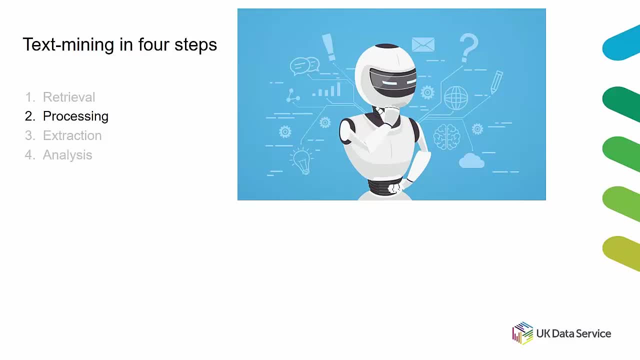 you will want to use computational tools. There's some very good off the shelf tools that you can use and adapt these, for example, in R or Python, And you will want to Become at least familiar with this if this is the step, that you're going to spend a lot. 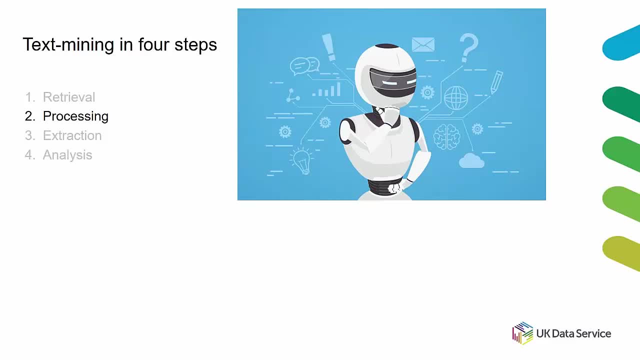 of time working on. So the practical steps of this include things like dividing and renaming files, So you'll take your raw data, download and maybe cut it into a series of documents that are one document per web page or one document per newspaper article, or one row in a data. 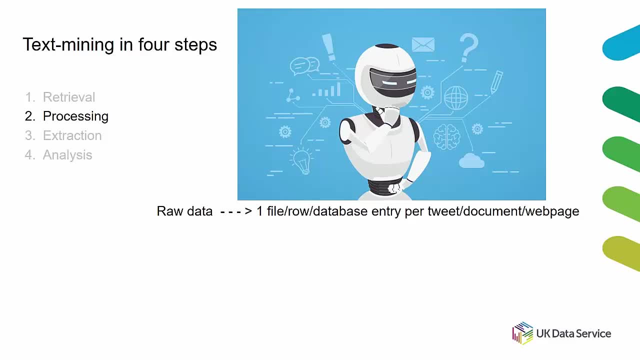 database per tweet, Something like that. So you want to cut it up into bits, And then you'll want to do sort of basic natural language processing, things like maybe correct spelling or remove capitalization or substitute acronyms or something like that, so that the 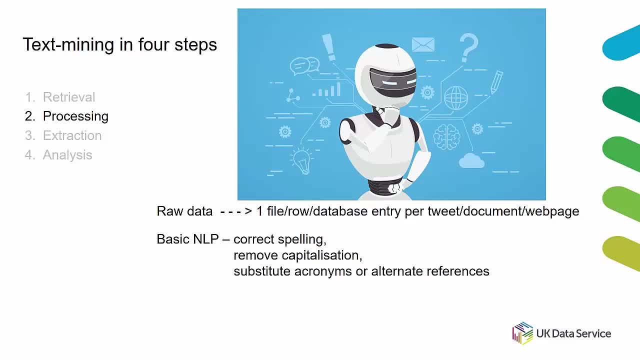 United Kingdom spelled correctly, or spelled with capitals, or written as the UK or UKGB or something like that, That those are all counted as the same, talking about the same thing, so that you have to sort of Process over it to make sure that the things you're interested in are counted properly. 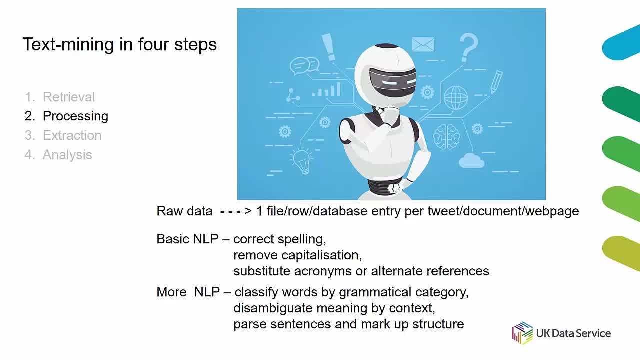 And then there's more advanced natural language processing as well, Classifying words by grammatical category, for example, disambiguating meaning by context and parsing sentences and marking up structure, And we'll go into the extract a little. this, a little bit in an extraction, because 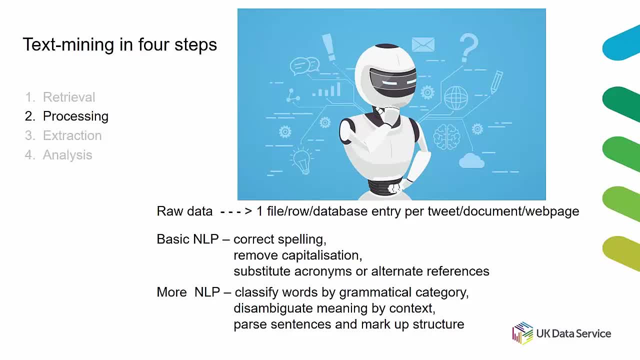 The processing step and the extraction step can sometimes Run into each other, and then you can sometimes need to loop back and forth between them a couple of times to make sure you know what you're doing, If you're going to do these steps on very large volumes of data, or are going to do these. 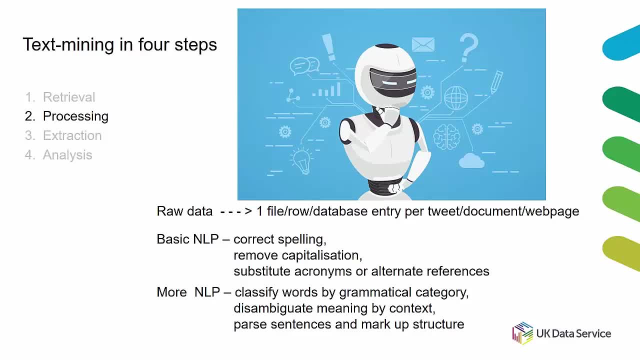 steps frequently on new data sets. you probably want to devise your own coding scripts to automate the processes, And that may require a lot of time at this point, But that will be time saved, Depending on the volume of work that you plan on doing with this kind of this step. 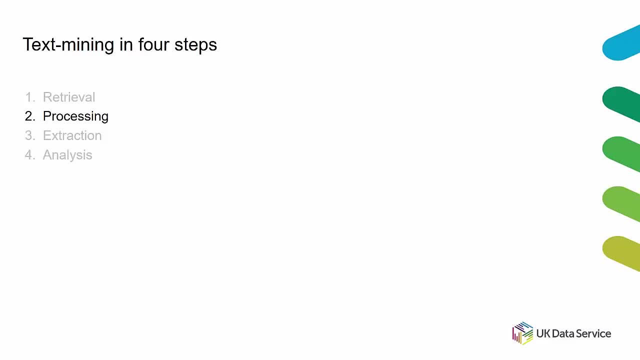 in the process. So extraction Is about running the analysis on the processed data. So, for example, if we are raw data, was this a sentence like this, maybe from a message board or tweet or something like that? it includes capitalization, punctuation and the 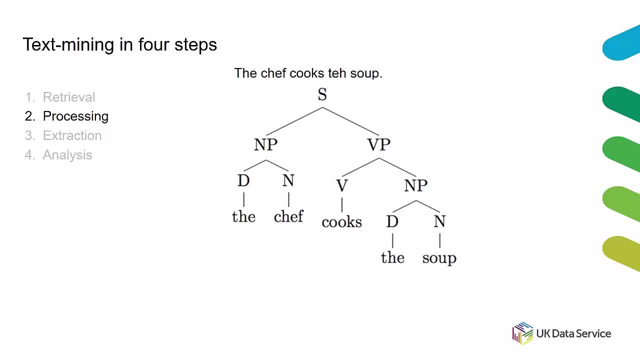 spelling error. We would process that To take out the capitals and the punctuation, the spelling error, And then we would put it genuinely into Machine readable Format, which here is sort of this nested set of brackets that have part of speech tags. and you know, definitive cook is is classed as singular and present tense, verb and things. 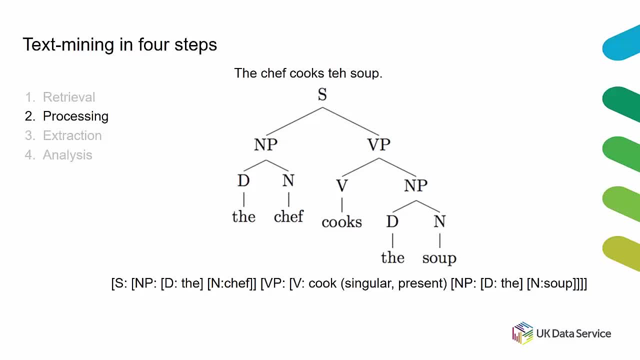 like that. This final sentence looks like gobbledygook to us, where we're much better as humans at reading the first sentence, despite the spelling error. But a computer is really going to need this, this sort of output, this nested series of tagged language. 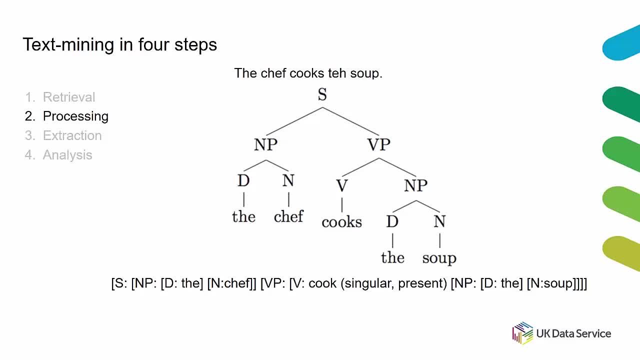 So this process does involve some choices. Do you want to remove the spelling error? Because maybe the top the research question that you're interested in involves not correcting spelling errors, Because maybe they're part of slang or they're part of part of the research topic that you're? 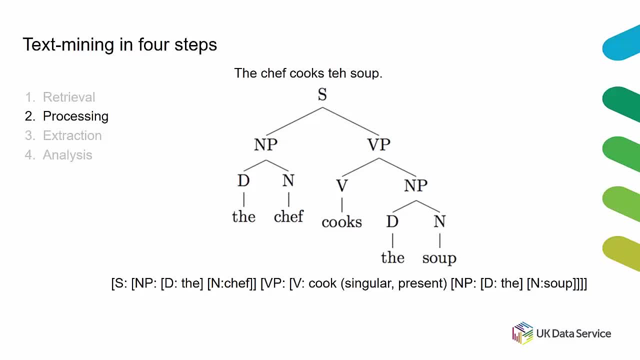 looking at in some way, But you'll want to document all the steps that you took. So did you correct the spelling errors? Make sure you say what, how you corrected the spelling errors and what program and at what step in the processing- that kind of thing. 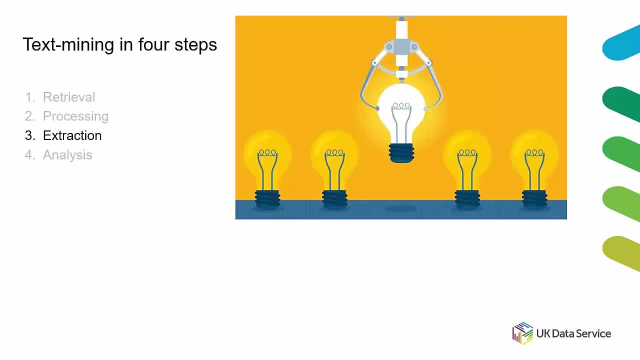 So moving on to extraction, Extraction is about running this, The statistical analysis and methods. This is relevant to your research question, So this might be fairly basic things like counting the relative word frequency of different words in your body of work, For example, people that write letters of support for candidates, you know job offers. 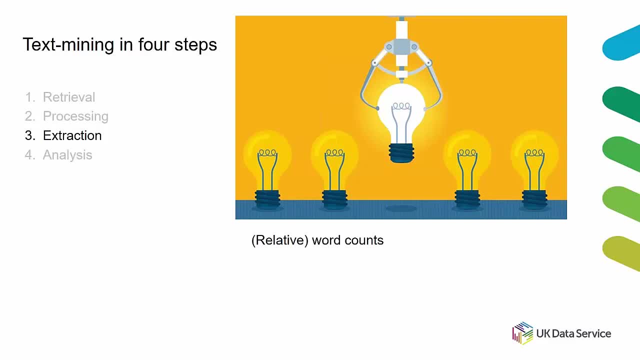 and that kind of thing. recommendation letters statistically use different words in different frequencies When they're writing about men or women Candidates. So this is the kind of analysis that, using something as very basic as relative word counts, you can show a statistical difference between letters written about men and letters written 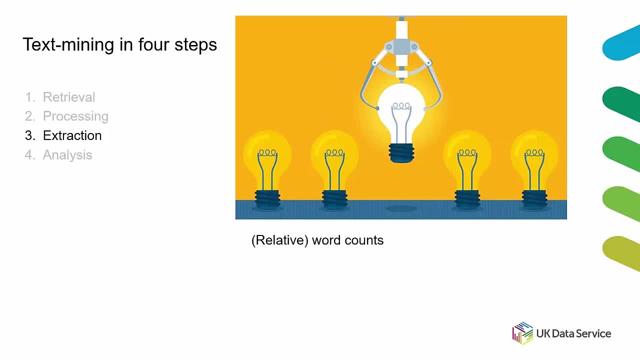 about women, But just the same, The extraction could be identifying patterns that are more complex than just relative word counts. So equivalency suggestions: You could show that how people use language Demonstrates that people are using two words in the same way but in different contexts. 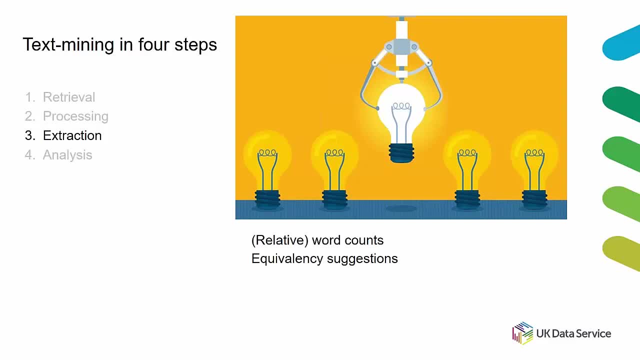 or the same word in different ways, in different contexts, and therefore that word has different meanings. So these are the kinds of questions that are a little bit more involved than just counting words, but they're also, you know, they're about counting and they're about counting. 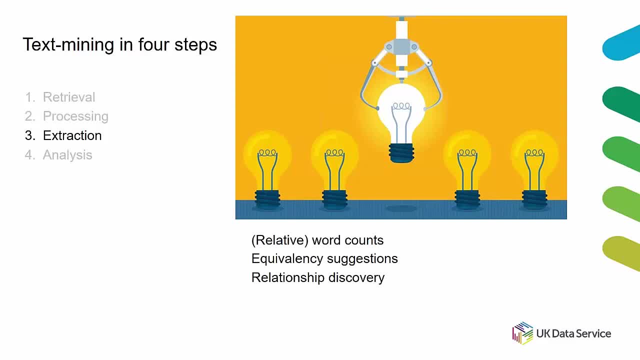 in context, things like that. There's relationship discovery. This one's quite interesting, Okay, So you could calculate the relationship between terms or entities or events or places or lots of things. For example, you could graph the social distance between people or between organizations based. 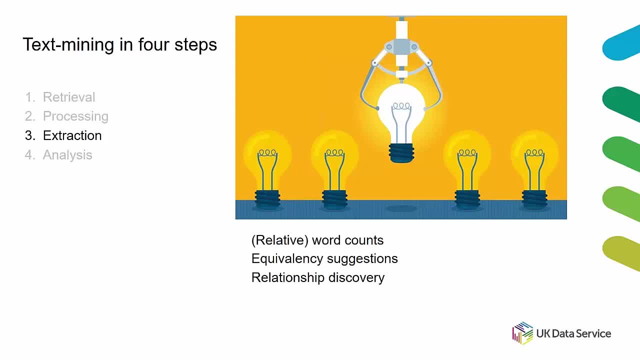 on how often they are or are not mentioned together in documents. You could put events extracted from a newspaper article into timelines or onto maps based on this kind of relationship discovery, because articles will say things like nearby Or previously, And you can use text mining to capture those kinds of words and turn it into maps of the 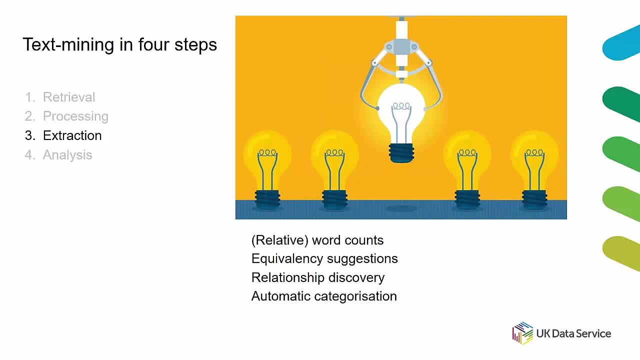 relationships between the entities. Automatic categorization: This is quite a popular one because it's a real time saver. It helps classify documents by sentiment or by topic, or by author or time period or gender. It can help recognize plagiarism. It can generate automatic responses to customer emails. 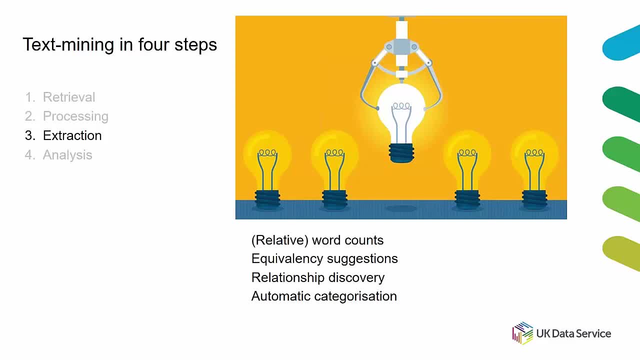 There's a lot of automatic things that can be done by getting text mining, sort of extractive processes, to look into documents or questions or tweets and recognize things automatically. And finally, prediction. This one is quite difficult, but it is also very interesting. 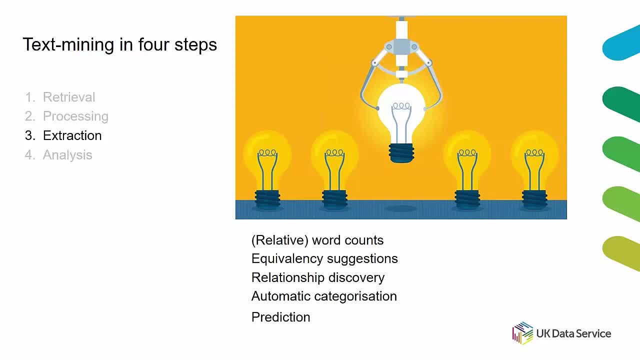 It's a growing area of application. A paper by Choi and Varian in 2012 referenced contemporaneous forecasting, or what they called nowcasting, to predict crimes or terror attacks based on intercepted communications. So they took intercepted communications as the data, they retrieved and they processed. 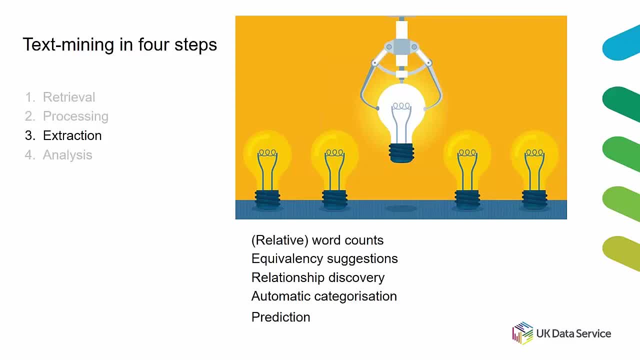 it in the way that they did and they extracted statistical sort of errors indicating that an event was more or less likely to happen at different points in time, And that's quite useful, potentially, if it's a very important event that you're trying to predict. 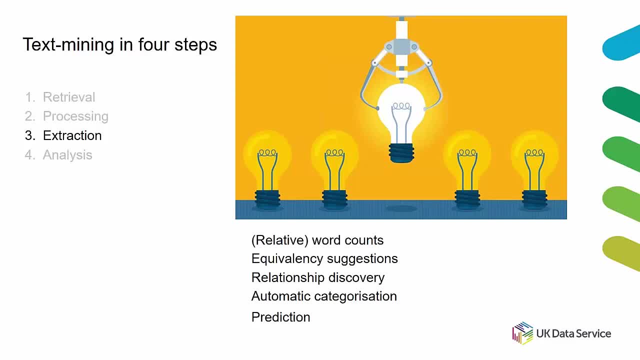 So all of these steps use familiar statistical analyses, more or less to show significant differences or significant relationships or significant factors of influence, And this step is more or less about your regression models and your p-values and your error bars and all the statistics that you're probably already familiar with. 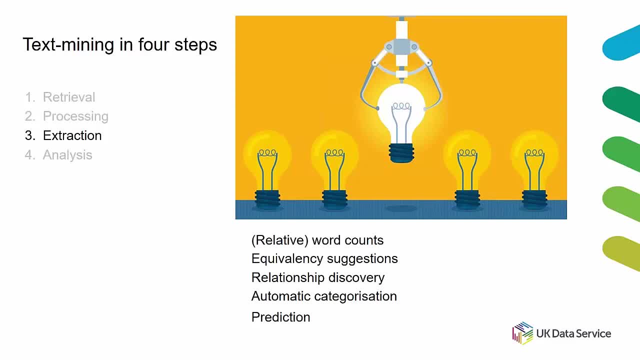 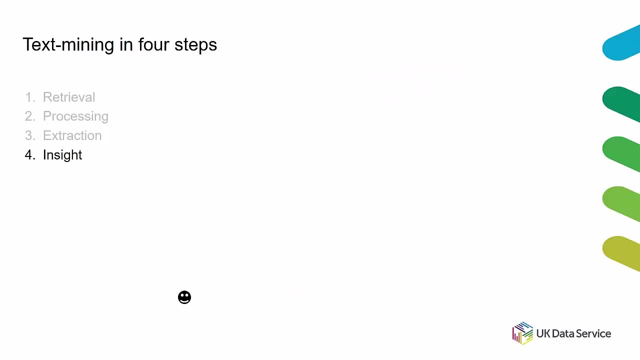 Exactly How they apply to text is perhaps less familiar. but yeah, that's just an application issue, We can learn that. And finally, insight. So insight, like step three, the extraction should be broadly familiar territory. It's about sort of showing the outcomes from the statistical methods. 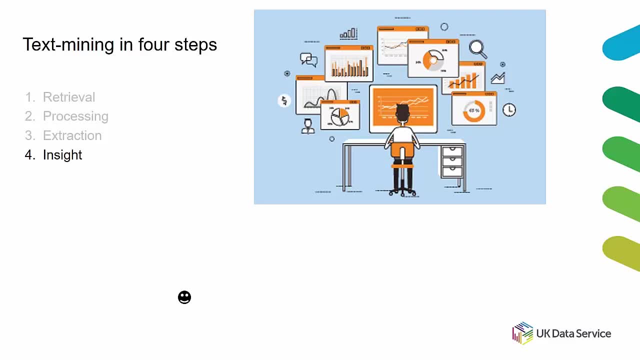 It also involves justifying all the steps you took, why you retrieved the data you did, why you processed it in the way you did, why you extracted the things that you chose to extract, why you ran the statistical tests that you did. And this will be quite familiar as a process to many of the hard sciences, because this 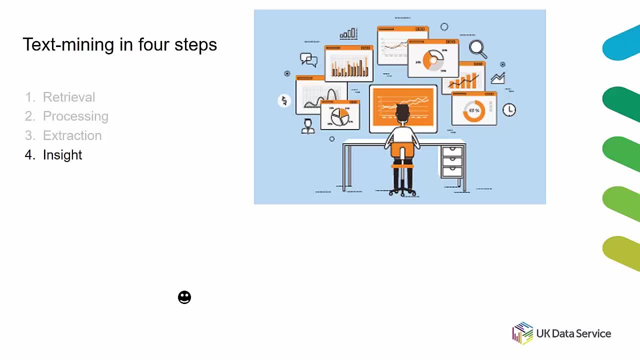 will be the methods section, it'll be the sort of results and discussion section and it's- You know, it's perhaps less familiar to some of the humanities. Social scientists are probably also familiar with a lot of these steps because they'll have to justify why they chose the sampling method that they chose or, you know, ran the. 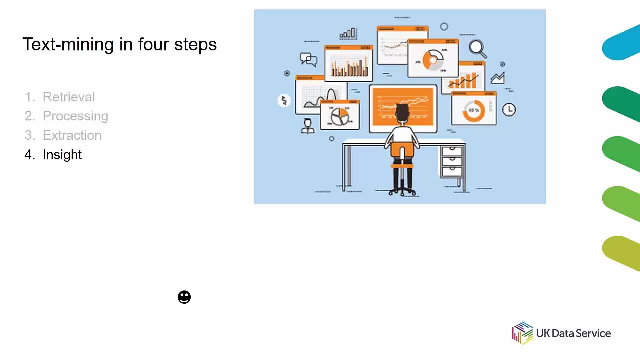 statistical tests that they did, But the more sort of abstract, expertise-based research. you know you can't just say, building on the theories of this previous person, we now add aspects of this. That won't fly. You need to be specific. 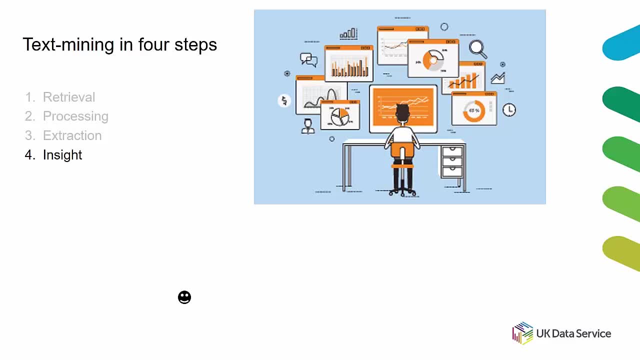 What theories are you building on? How have you added to them? Why have you added to them in the way that you have? So this step also includes presentation or visualization of your results, which can be very difficult when there are not as many well-accepted examples how to present or visualize. 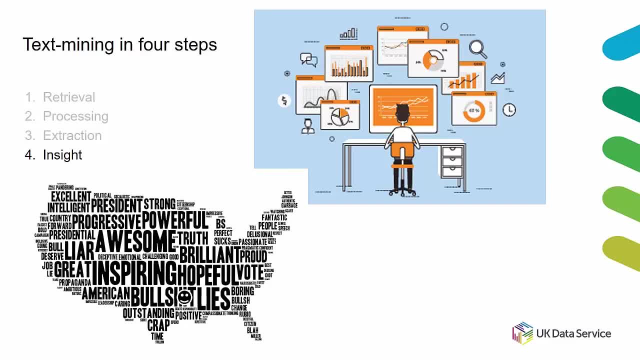 those results. For example, this is a word cloud of one-word reactions to one of President Obama's State of the Union Address. The size of the word represents frequency. Okay, So this is a word cloud of one-word reactions to one of President Obama's State of the Union. 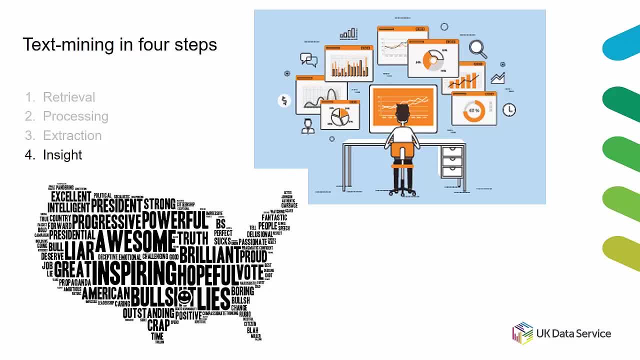 Address. The size of the word cloud represents frequency, But location on the apparent map is irrelevant. Now, this visualization is a very different impact than you would get with a simple table of the words in one column and the frequency counts in the next. 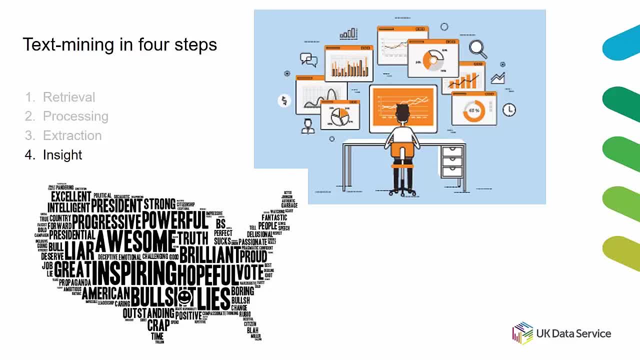 It is. you know it has a very different impact, but you have to be prepared to consider that maybe that impact could be misleading, because people might interpret the location of the word as being relevant to where the people who used that word were from and that's. 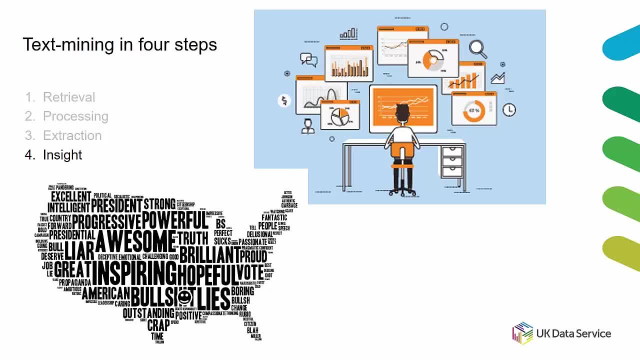 not accurate in this case. So is it useful? Is it misleading, Is it distracting, Is it just unfamiliar? Is it perhaps quite encouraging because it shows very visually, you know, something that's very hard to do with a table? I mean, probably people would not look at a table nearly as much as they would look. 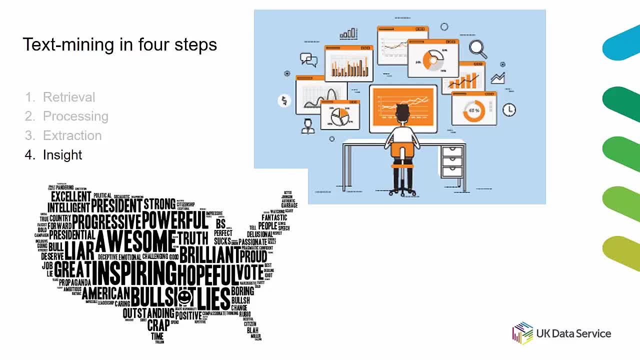 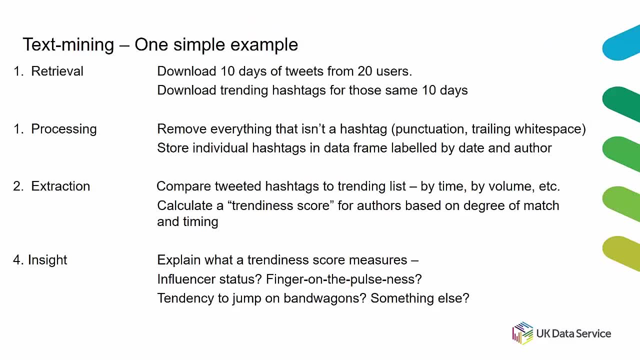 at an issue line, A visualization like this and that's useful potentially. Oops, Let me just seem to have an error in my animations here, but I'll just walk through all four steps of one text mining example that I did consider. 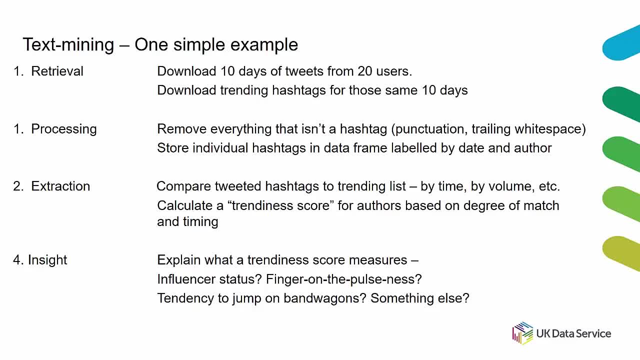 So, for example, if I wanted to download 10 days of tweets from 20 users and also the trending hashtags for those same 10 days, And I remove everything that isn't a hashtag and I store individual hashtags in a data frame labeled by date and author. 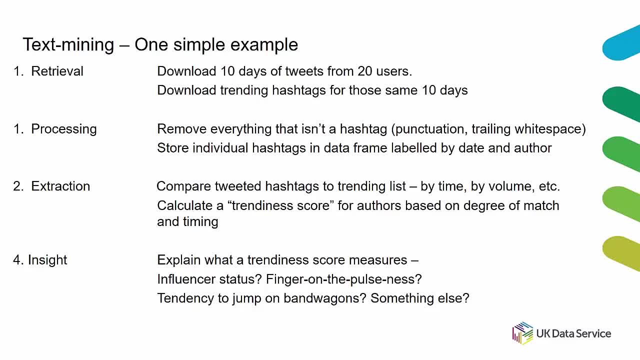 Now I want to compare the tweeted hashtags to the trending hashtags. you know to calculate a trendiness score for authors based on the degree of match between the trending hashtags and their tweeted hashtags, and also the timing. So my insight would be about: you know, what does this trendiness score indicate? 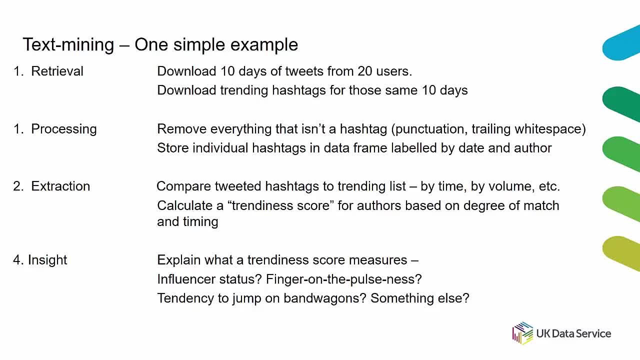 Does it indicate? Does it indicate someone is causing hashtags to trend or that they are quick to react to hashtags that are starting to trend? Does it indicate that they follow trending hashtags quite closely and that they start participating in things as soon as they become trending? 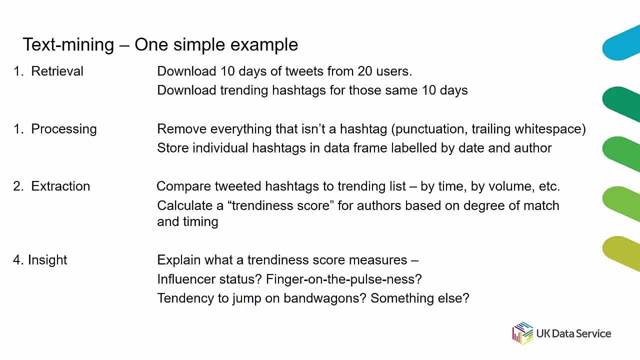 Something else, Just to let you know. I did not actually do this bit of research, but this is the kind of research you could do if you had a research question about how do we demonstrate that people you know cause hashtags to trend or respond to trending hashtags? 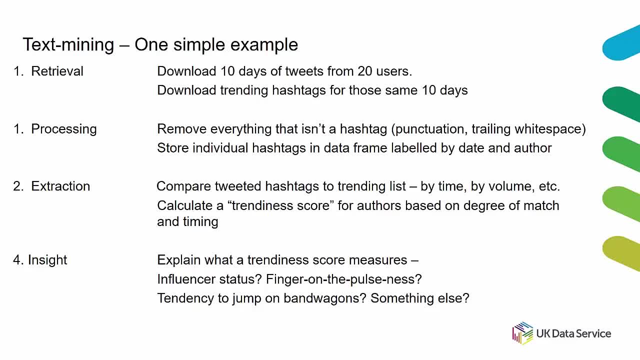 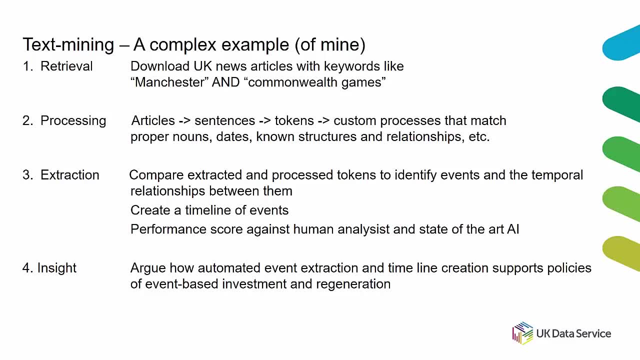 If you had a research question like that, you could do these steps. Now, a more advanced example, and one that I actually did participate in, was to download news articles with words like Manchester and Commonwealth Games. put that through some very extensive natural language processing. 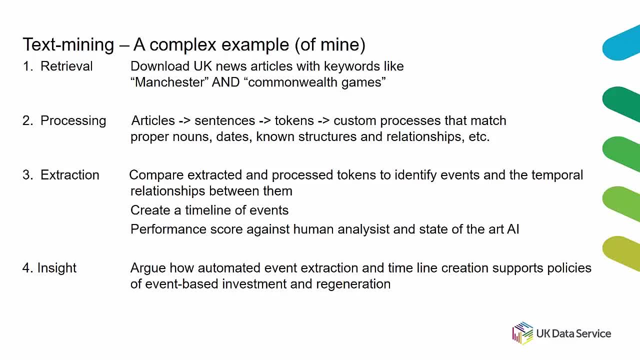 To pull out the nouns, dates and known structures and relationships and then compare, essentially to create timelines of events about when investment went into an area in order to host a mega event like a Commonwealth Games, and what kind of regeneration events occurred after. 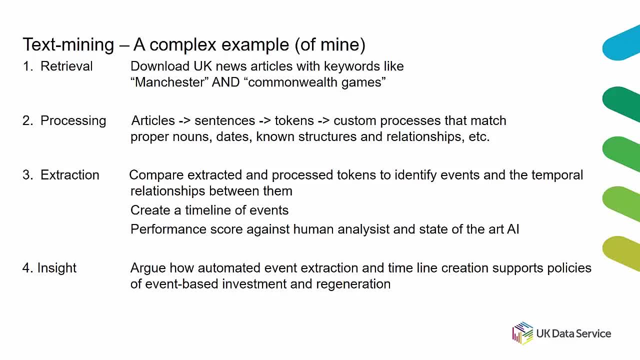 and like long after, 20 years after. So we did a timeline and one of the outcomes of this research was to compare whether we could do this automatically better than people could do just actually reading all of the articles and scoring things. And it turns out we did okay, but it was much faster than people. 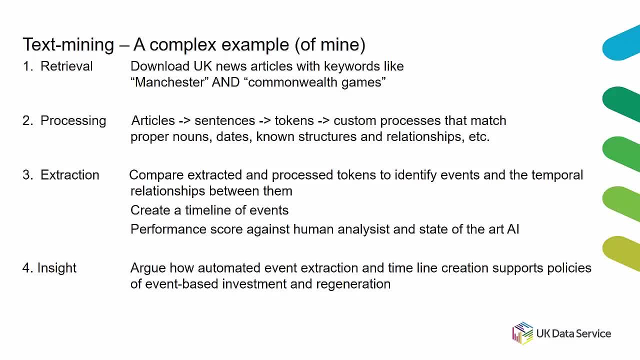 So you know there's a bonus there. The insight was about whether we could use automated event extraction and timeline creation to support policies. So that's kind of how investment and regeneration around events go together. So feel free to ask me more questions about this at the end if you'd like. 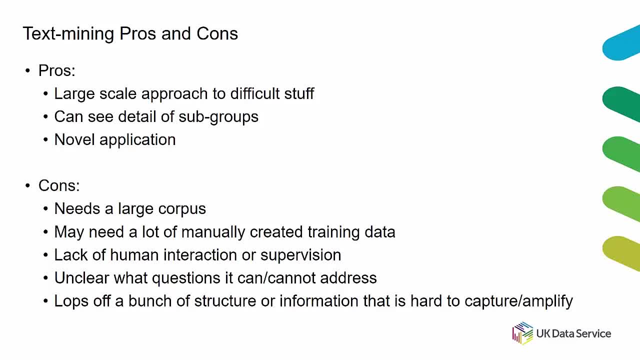 Every text mining choice has pros and cons And text mining in general has pros and cons which I did address there a little bit. You know you need a large scale. it's a very large scale approach to difficult stuff. We are really not going to get traditional sort of humanities exercises. 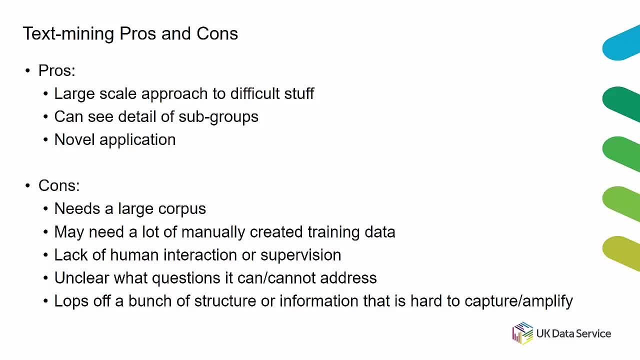 We've got to be really, really focused on the basic part of science. So that's the first thing I want to show you is that text mining has pros and cons, And text mining has pros and cons. It's really important to know when to get started. 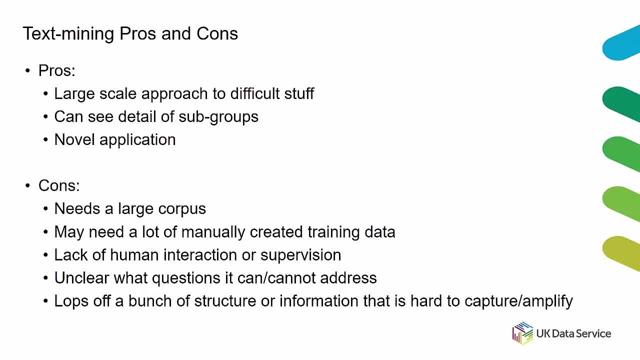 And I'm working with a lot of experts to read thousands of newspaper articles looking for tiny little details like whether you know businesses closed just after you know the stadium opened, or whether they relocated, or whether they opened closer to the state. 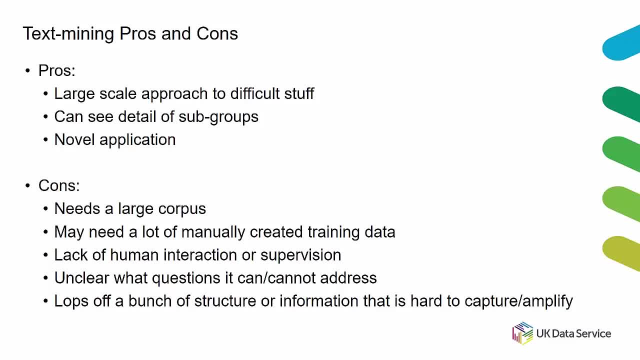 You know that's the kind of tedious detail that is not really worth the time of. you know really critical thinkers, But it is the kind of tedious detail that computers do. computers are happy to spend their time on and because it's such a large-scale, 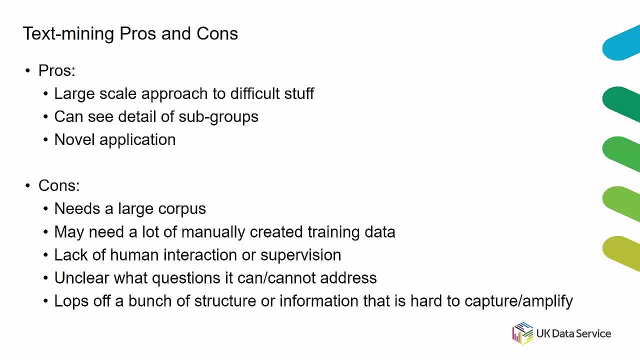 approach to really tedious, difficult, boring stuff. we can get into details that would not be accessible if we tried to get real people to read all those things, and we can support novel applications, like you know, trying to predict criminal acts or trying to, you know, justify different kinds of policies. 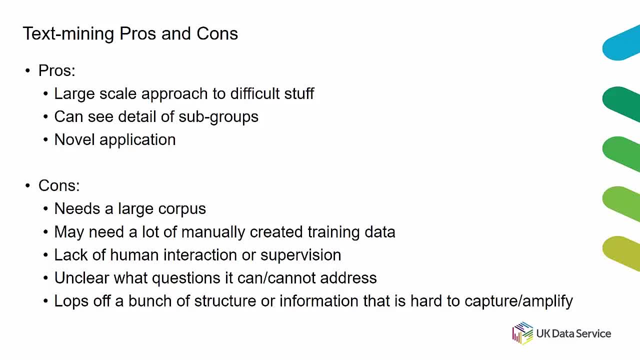 that so far people have not necessarily been able to justify their decisions very well. on the negative side, you do need a lot of material and not all of the topics that people might want to. not all the research questions that people have can be matched with a large enough body of material. also, you may need a lot. 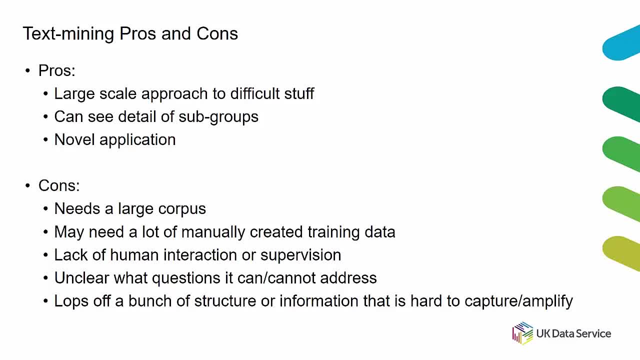 of manually created training data. that is something I haven't gone into but we can talk about at the end if you're interested in how that process goes, especially if you're going to run a process on huge volumes of data or run a process multiple times for quite long time frames, you know, if you 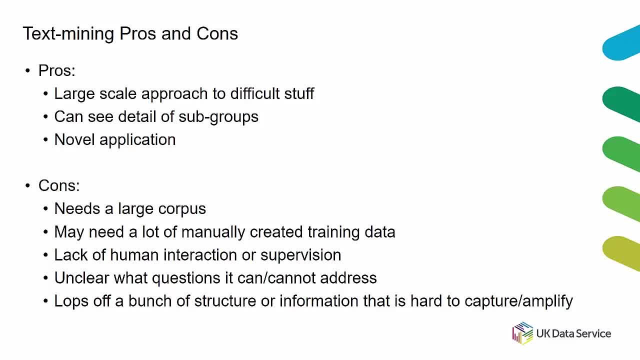 want to every single month analyze the previous month's tweets. you're gonna want a lot of manual work to go into the automation process. there is a lack of human interaction and supervision, so it's not always easy to say, when the computer comes out, something. sometimes it can be hard to believe and sometimes it can just be hard. 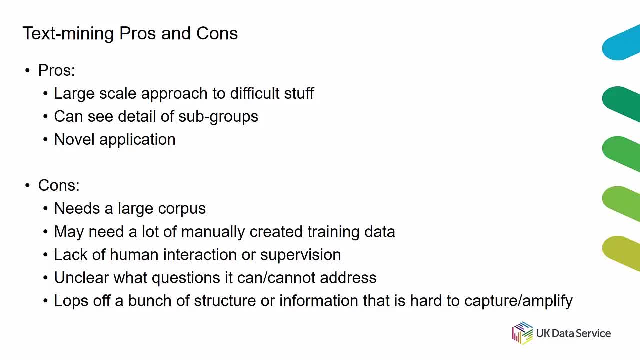 to interpret, and so far because- partly because this is new- we're not clear what questions text mining or or the data mining processes are useful for addressing. so it might just be that people are trying to apply text mining to questions that there are other or better tools for, and another issue is: 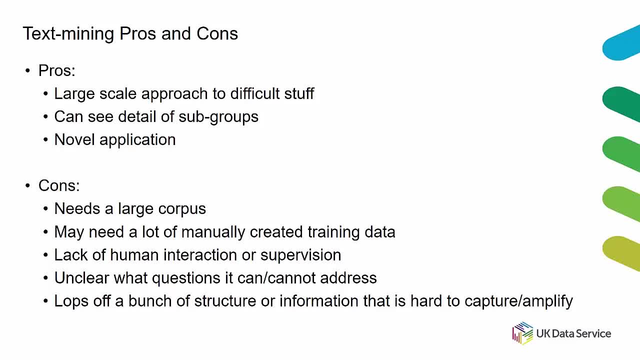 that enforcing semi-structured data into a more rigid, coherent, uniform structure, we do cut off some of the information and structure that is hard to capture or amplify. so when we correct spelling, for example, we make it easier to count instances of a word, but we lose out on the fact that maybe some people are using words ironically or you know as. 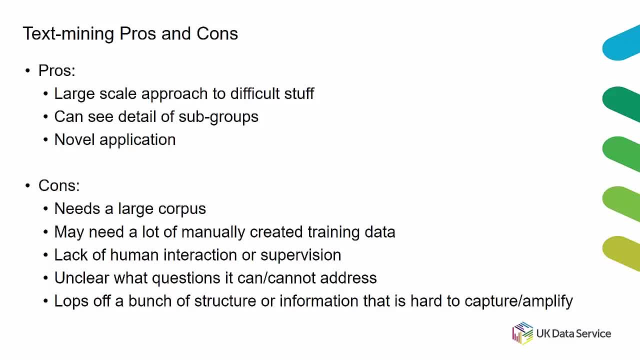 slang or in new ways, or that they're more likely to be used by people who are using mobile devices as opposed to keyboards or something like that, and that that information is harder to think about and capture and amplify. it may become important. it may not be it kind. 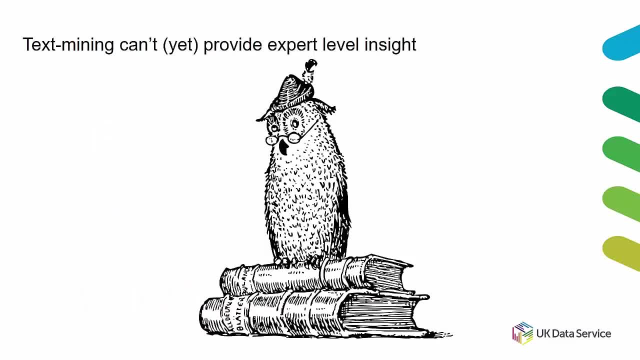 of depends on your research question. so it is very important to show that text mining cannot yet provide the expert level insight that a lot of people are having and that's something that a lot of humanities research has. you know, text mining, even though it can read all of the books in the library, it will not be. 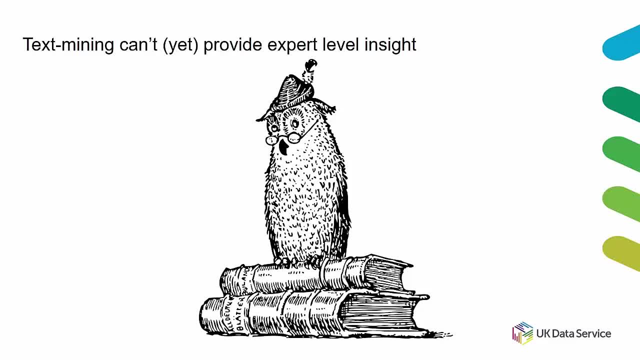 the same. it will not have the same expert level insight afterward as a human who had read all of those books. it just won't work. you know. there's just that's like saying that you know, if a text mining sort of algorithm processes a book and tells you how many, 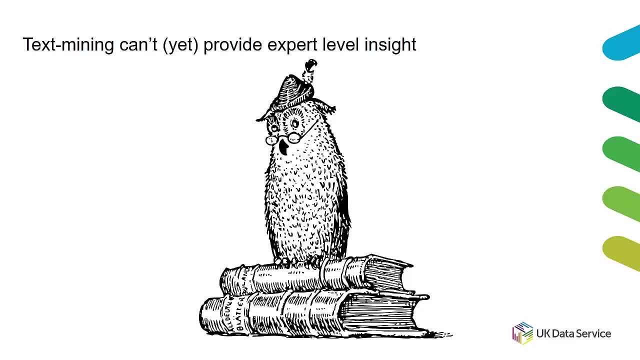 counts of the word is required to determine your current text mining data. the are in the book. that's not the same as the human who writes a literary criticism of the book or something like that they're. they're very different process and they don't cut the same output, which is fine because text 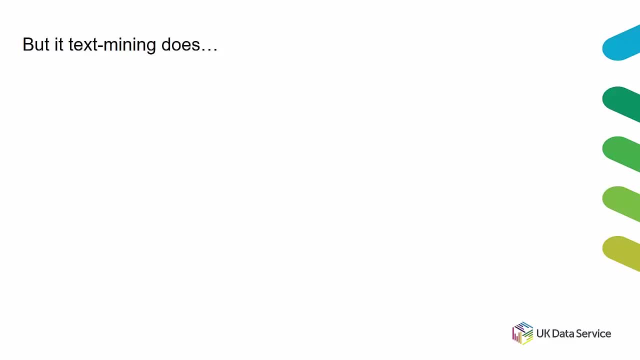 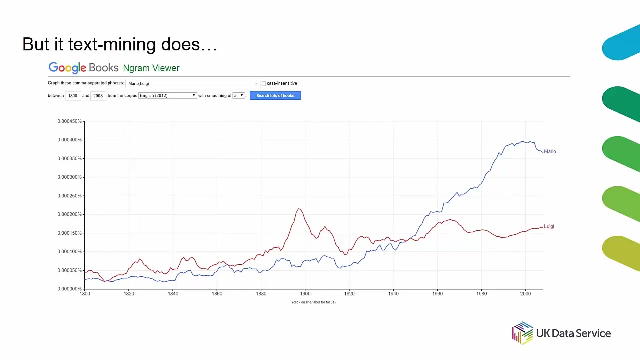 mining has other benefits. it does very quickly sift through a whole lot of data, and it can it can help you notice interesting things that you can then apply your expert level insight to. so for example, just as a bit of a lark, I searched for whether Mario or Luigi, you know, plotted on Google Books n-gram. 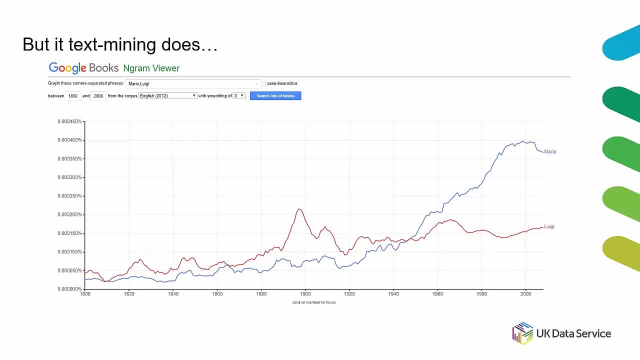 viewer. so this shows how popular these words were in all of the books that are in Google's history over time, and we see that they're pretty close. for a long time, Luigi has a good spike just before the turn of the 20th century. go back to being close. 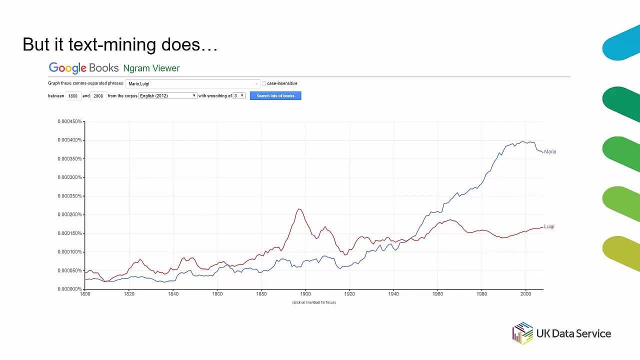 and then you can see that they're pretty close. for a long time Luigi has a good spike just before the turn of the 20th century, go back to being close and then Mario takes right off in the 50s and Luigi is left behind. so this is not a 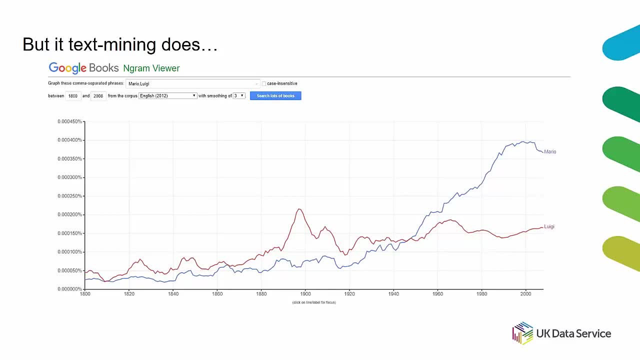 research question that if I had to read all of those books I would not be interested in producing this graph manually. but I'm happy to produce it through n-gram viewer and other text mining methods because it is quick and easy. is it worthwhile? that is difficult to say, but it does show that something. 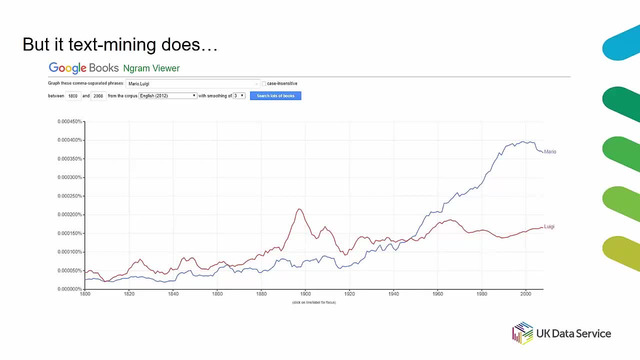 happened before the turn of the century that made Luigi much more popular, and that something happened in the 50s that made Mario much more popular. so you know, we can use text mining in this case to find patterns that are worth exploring through other methods, maybe even other text mining methods. but you know it's 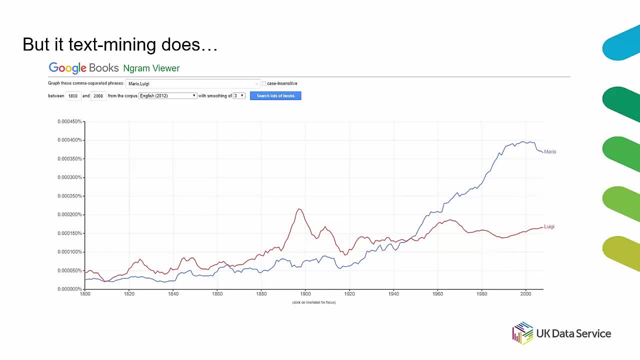 the fact that it's automatic and it's easy and it's fast is very, very useful for pointing us towards more interesting research questions to approach. yeah, we're also, you know, less interested in How To Minimise The Maths and Read More, less likely to waste a whole lot of time.